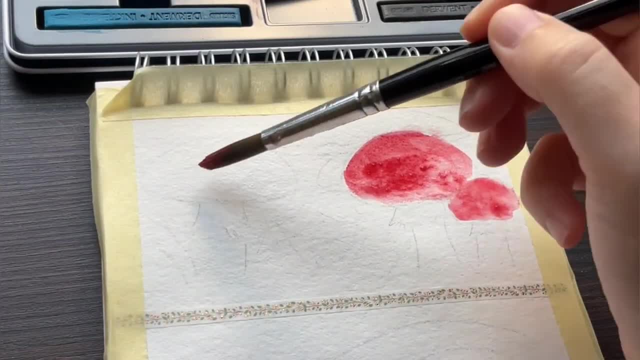 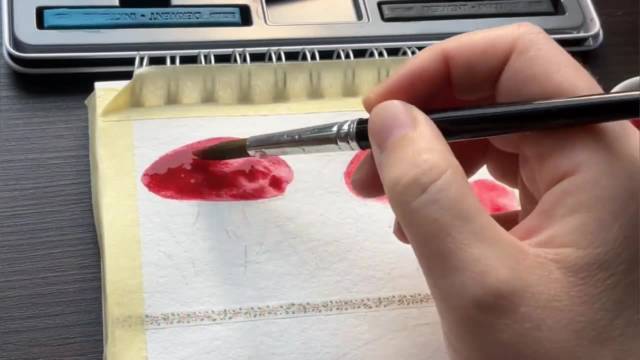 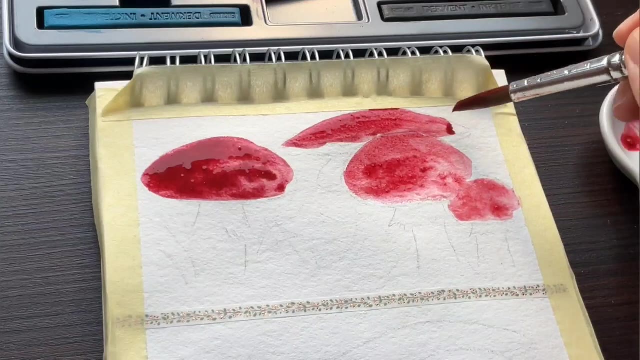 blocks and the XL blocks. I'm going with the regular ones now. They are basically an ink-based, water-soluble pastel medium that can be used in various ways. They can be diluted and applied as watercolors. they can be used as dry pastels, as watercolor crayons. 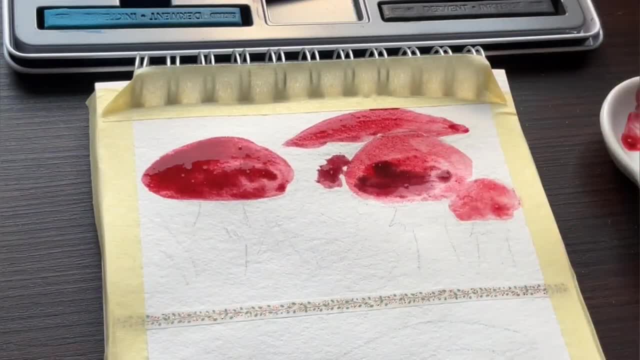 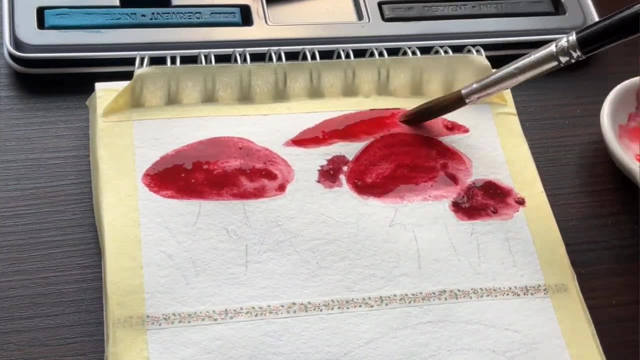 They work on a number of surfaces, including fabric. No wonder they are so popular. but they're also kind of misunderstood, I would say. A lot of people seem to be disappointed with them, I think, the main reason being they can't really find out what to do with them. 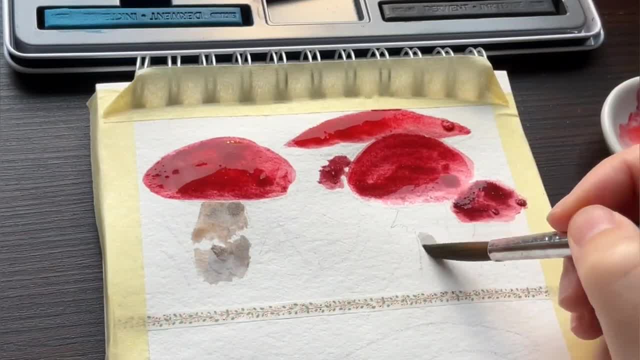 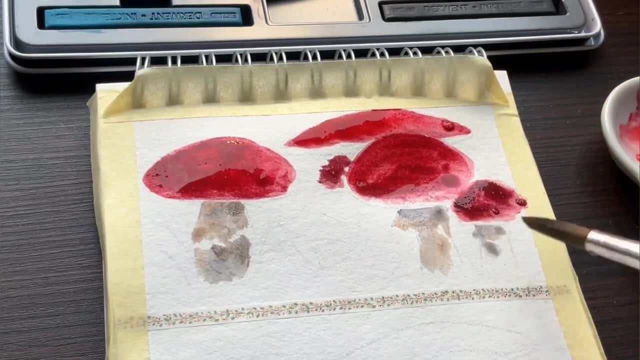 or they simply just expect them to be traditional gum. arabic based watercolors which they are not Painting with Inktense blocks is challenging at first. Paper is extremely important. I have a separate video dedicated to this topic in the description box. If you're interested, you can. 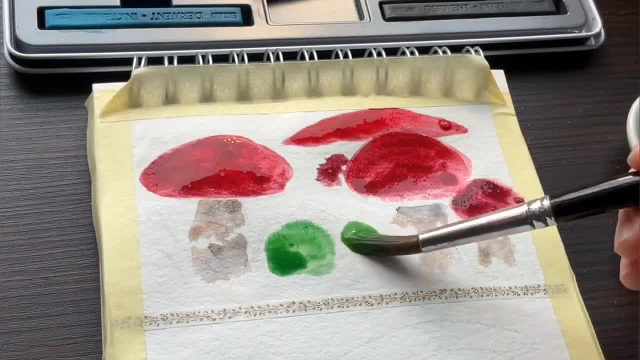 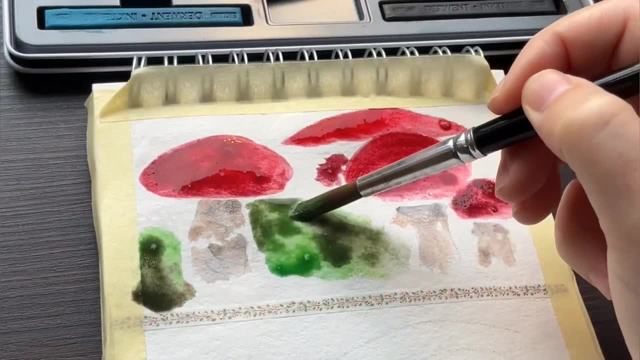 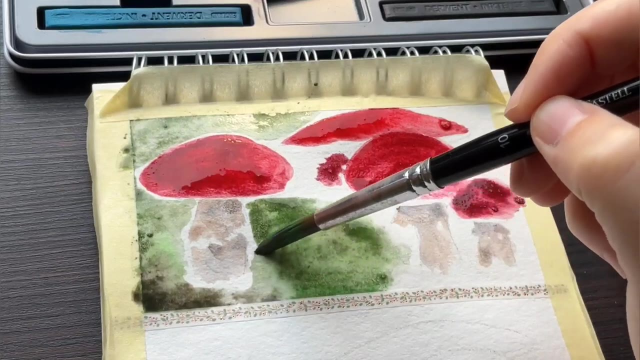 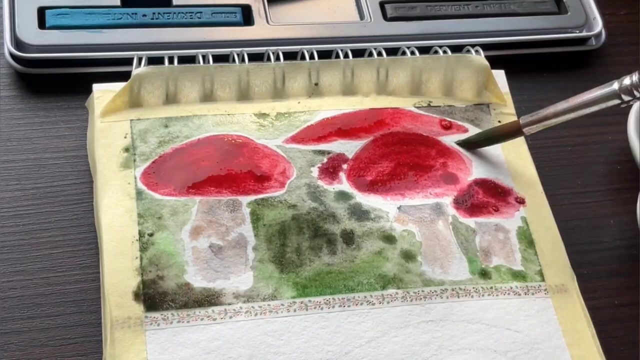 find it on my Inktense blocks playlist. But even choosing the right paper, it really takes some time to get it right. One of the things to deal with is almost every Inktense blocks painting has an un-painted surface. So if you're looking for a paper that's not completely un-painted, 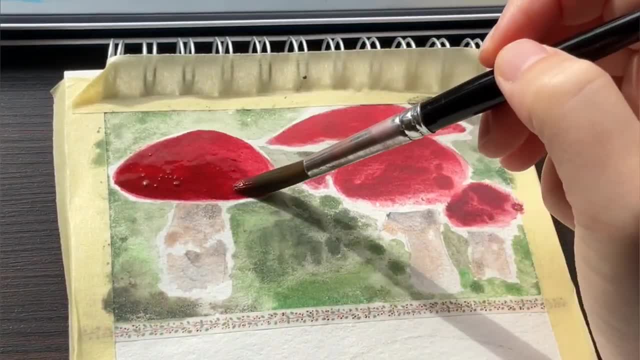 you can use a paper that's not completely un-painted. If you're looking for a paper that's not completely un-painted, you can use a paper that's not completely un-painted, especially when you're not using 100% cotton watercolor paper, and I'm purposefully not doing that here. 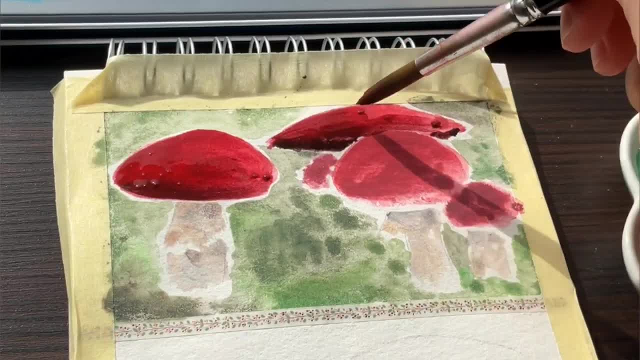 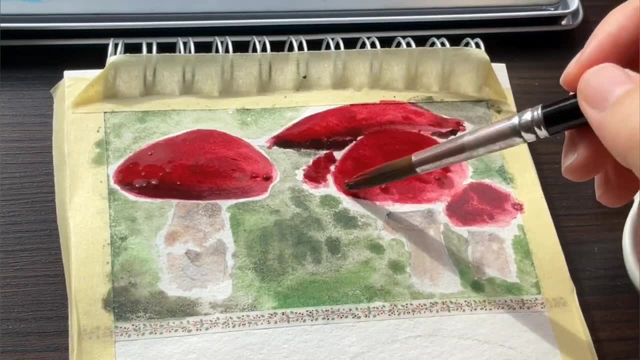 This medium is made out of ink and a chalk-like water-soluble binder that may occasionally look chalky, especially on cheap paper. It may also appear streaky and patchy, which can be really disheartening. It doesn't bother me much because of my mixed media. 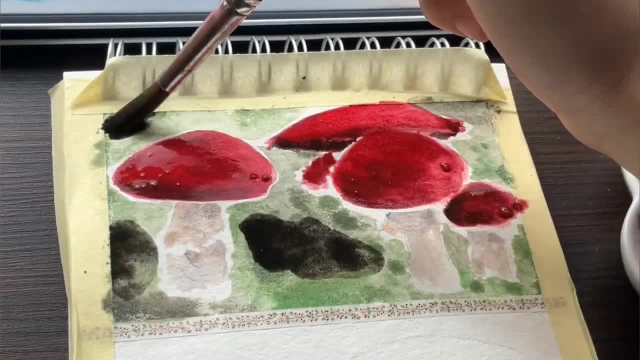 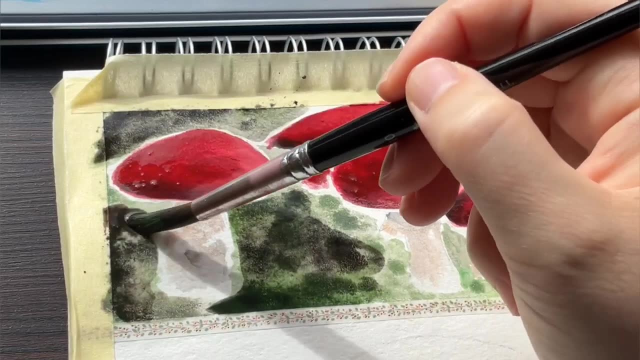 approach to painting in general, but I know that people are let down by it, so that's why I'm addressing it here. For completely smooth, non-streaky effects, I obviously recommend 100% cotton paper because it gives the best results with Inktense, but a more budget paper can also. 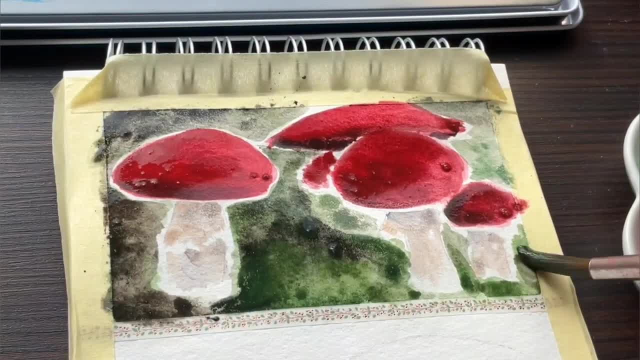 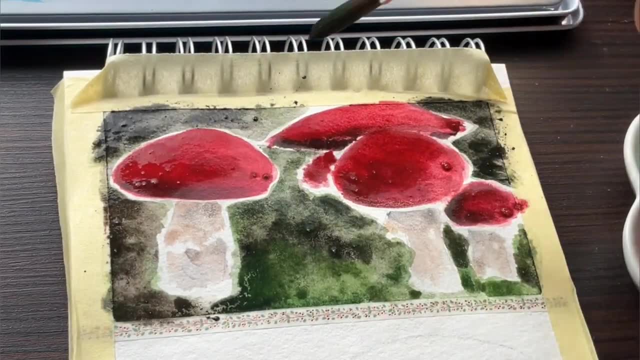 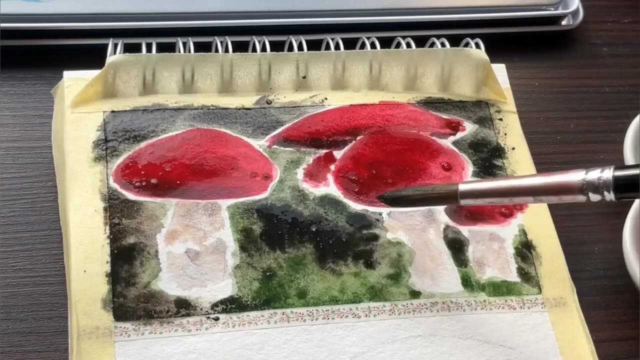 work really well for thicker applications and a combined use of wet washes and the dry pastel effect on top. This painting is exactly that. First, I'm putting down at least three wet layers which will give me a more opaque, almost gouache-like watercolor effect, which soon 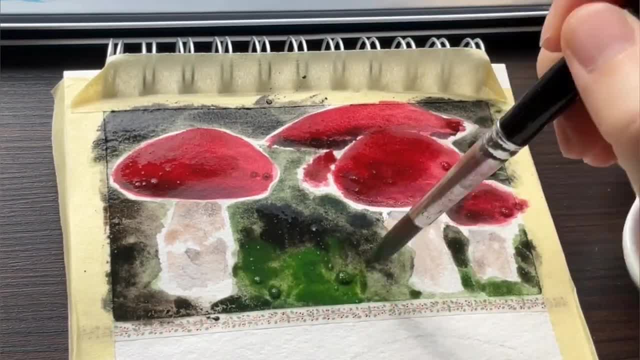 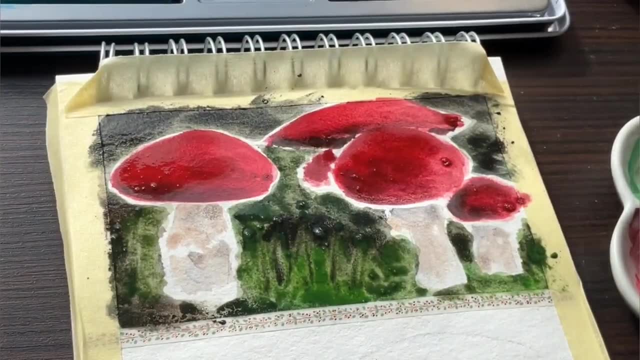 will give me a super vibrant color and a lot of depth. I like to use a lot of water in my paintings, and one thing that I really love about Inktense is I don't have to worry about cauliflowers because the particles are just way too heavy to bloom, And I love. 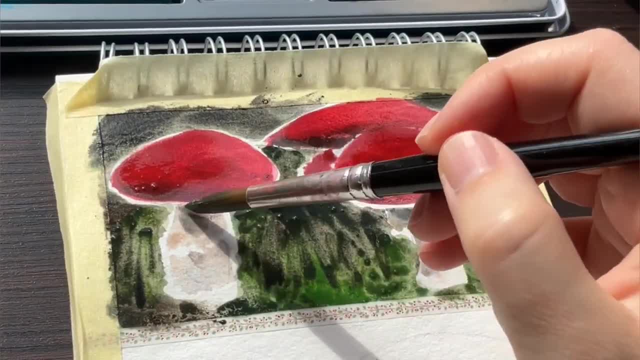 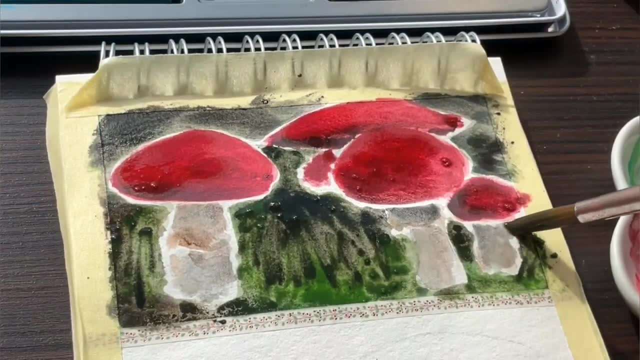 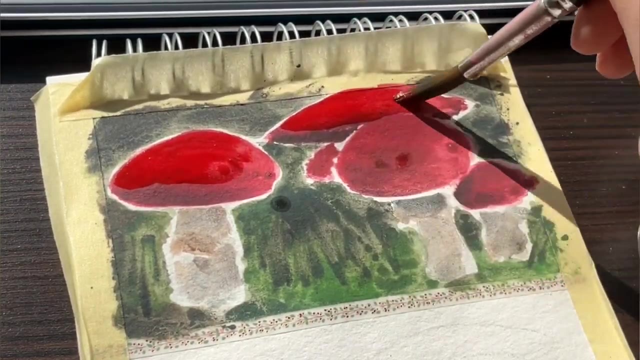 love the fact that the layers stay put and I can add as many layers as I want without destroying or overworking my painting. Inktense is actually a very forgiving medium And you may ask yourself: how am I going to go around my painting without 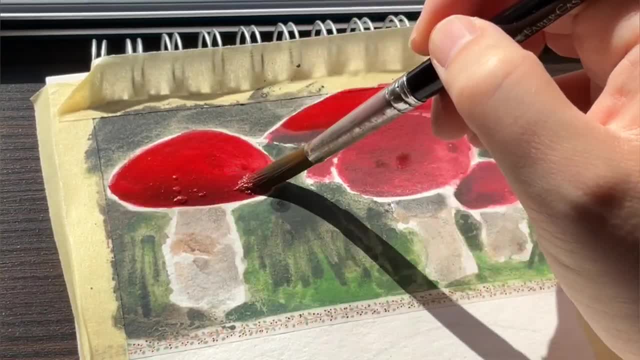 having too many layers of water. Well, I do this for the sake of this painting, So I'm going to be doing a few of these layers a lot. I will be showing the more subtle layers here in a few minutes. So I guess that's basically it for this painting. 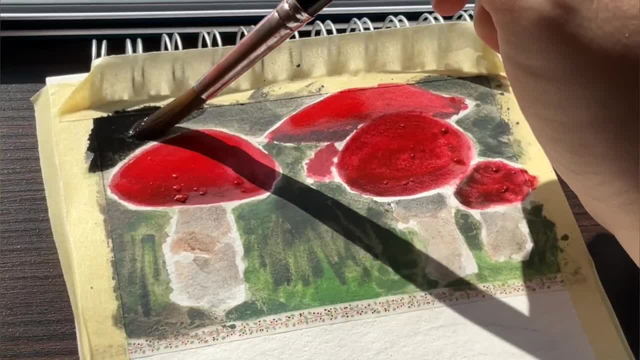 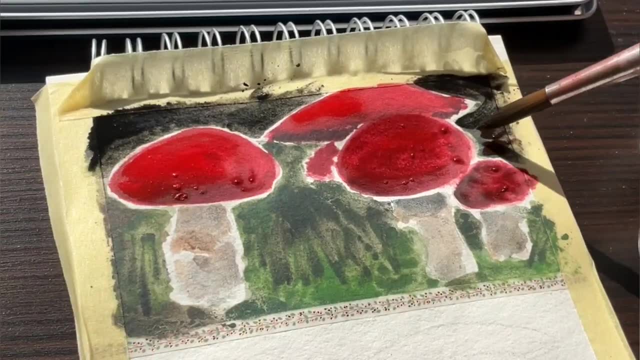 I've already painted the top layer and now I'm going to show the top layers, Because this one, I'm painting the top layer with a thinner layer of water. By doing this, I'm actually bringing out the whole, the metallic, the matting layer of the layer. 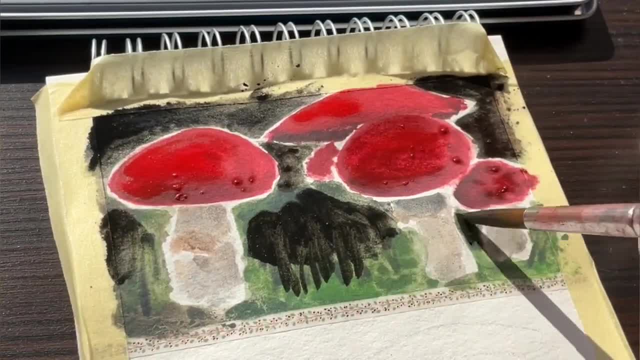 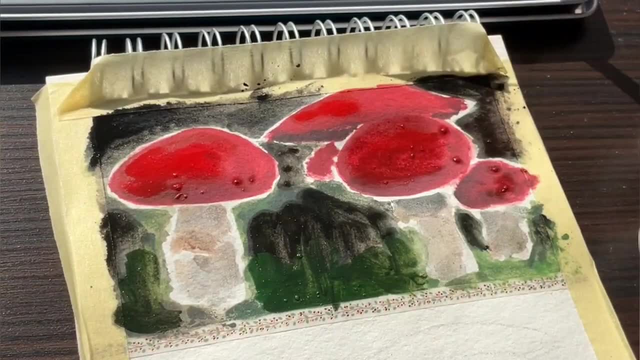 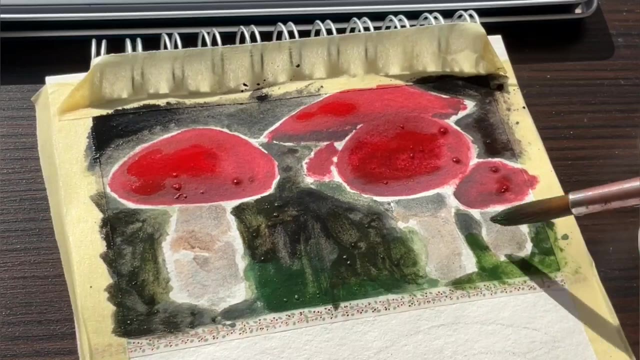 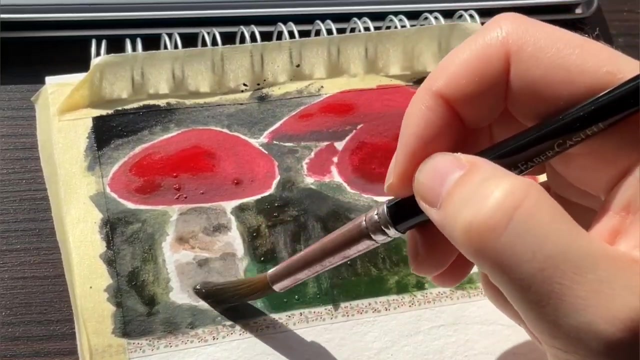 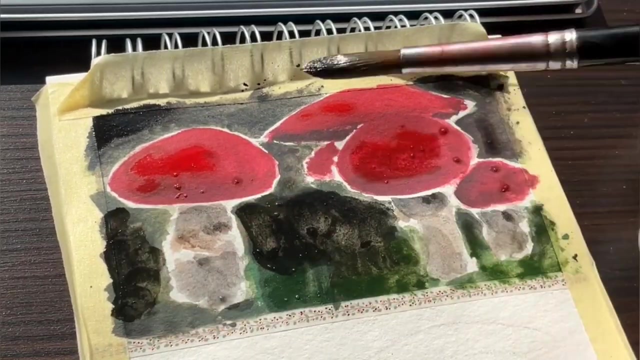 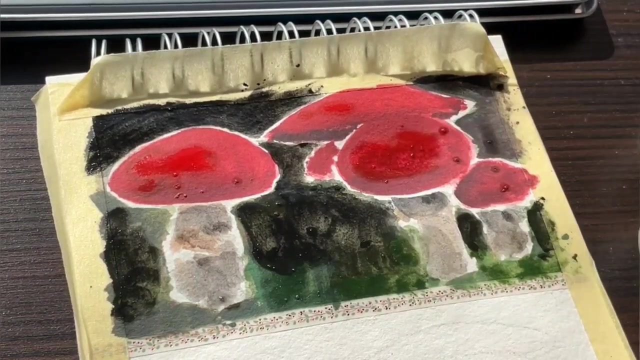 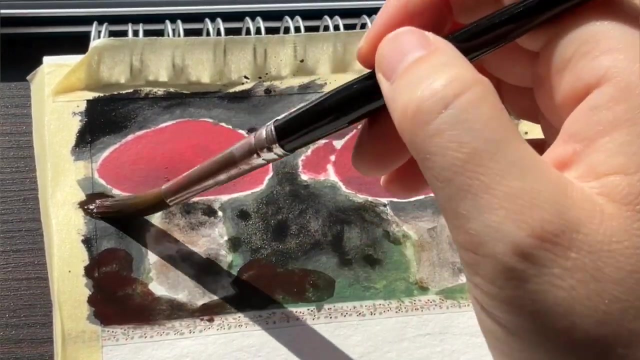 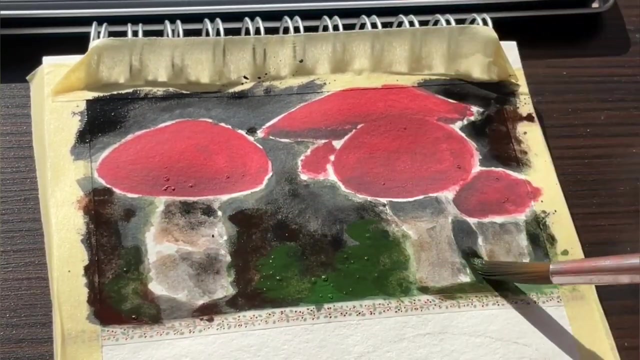 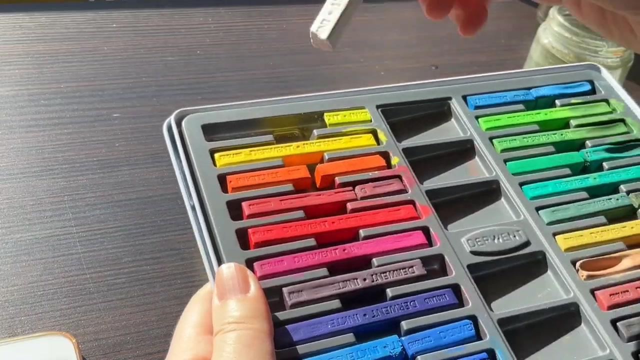 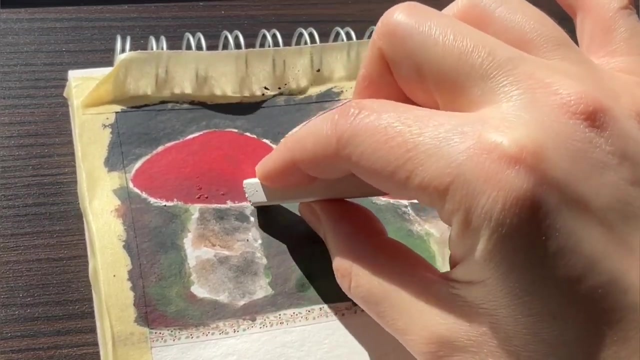 Thank you. Okay, we are done with the underpainting. It's time to use the blocks as best styles, which is kind of the bonus feature of any similar medium as opposed to traditional watercolors. I'm dipping the white Inktense block directly in. 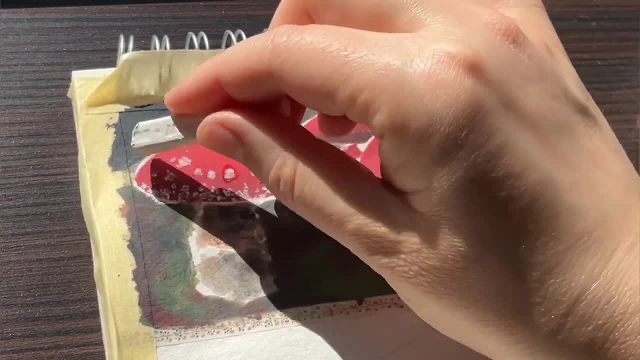 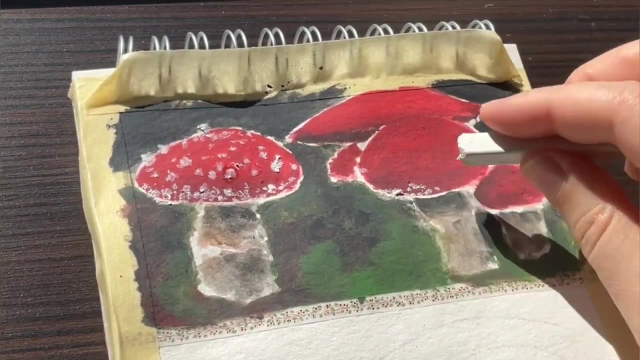 water to activate it, and that's how I'm going to create the white dots on the mushrooms. The Inktense white is very opaque, which can be super handy in like winter landscapes and so on. The white also comes in XL form, but I really 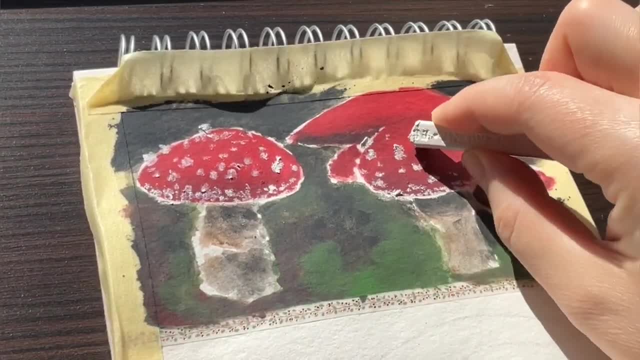 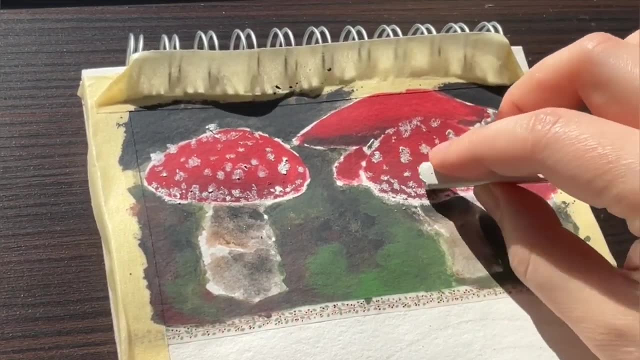 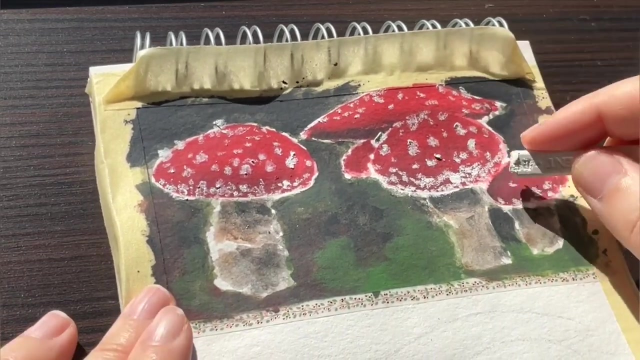 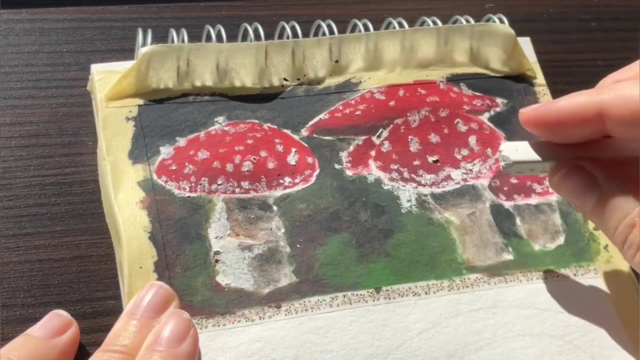 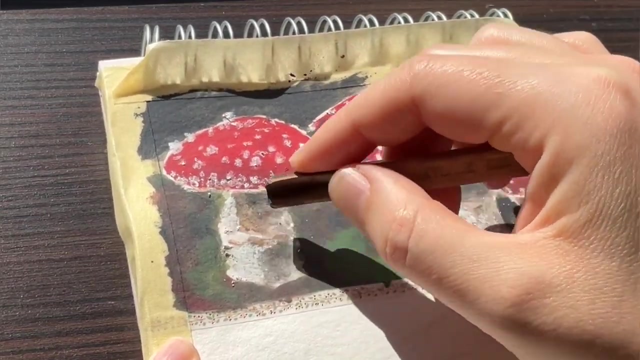 enjoy using the small one for details At this stage. I'm slowly switching to using the blocks completely dry, as I would draw with chalk pastels on top of gouache or watercolors, And the result is, I think, a beautiful mixed media effect that I want to practice. 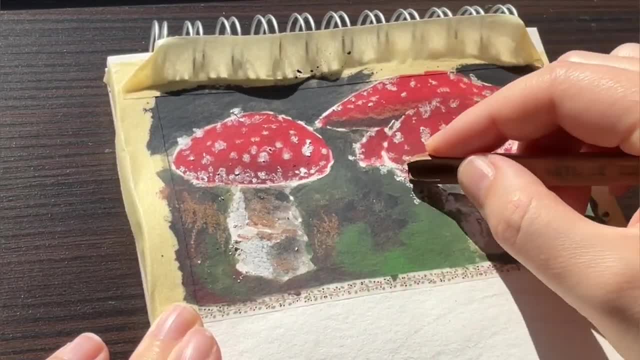 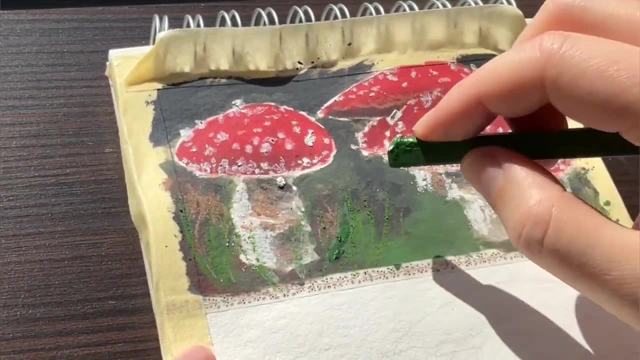 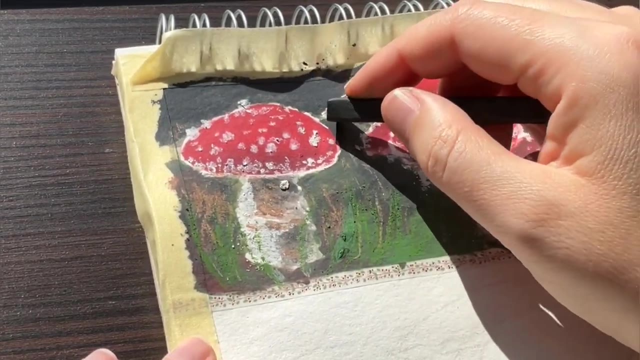 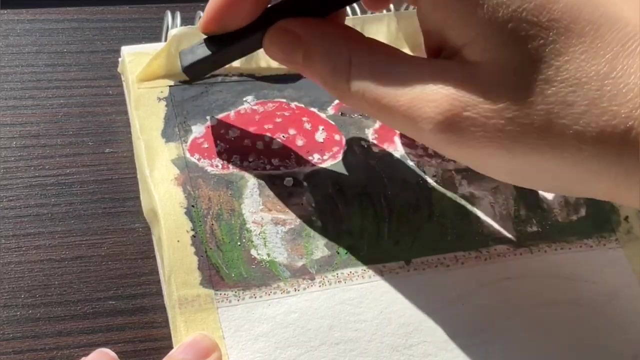 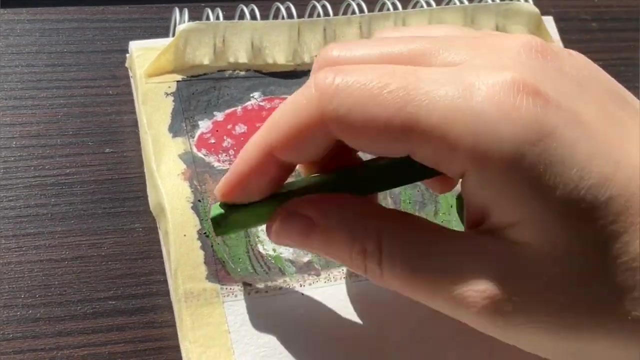 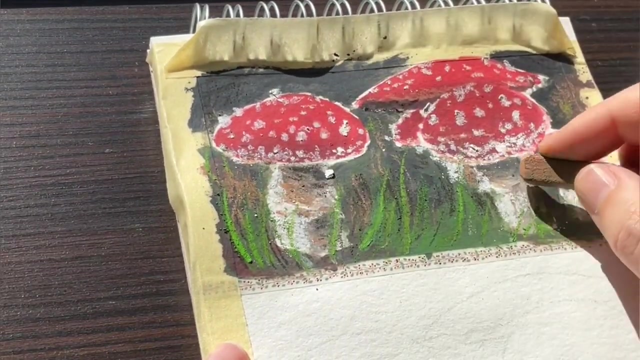 more this year. The more I use these blocks, the more versatile they become in my eyes. They're great for painting. If you've got a question you'd like answered about what I use and how to use them, I've got a lot of questions in the comments. 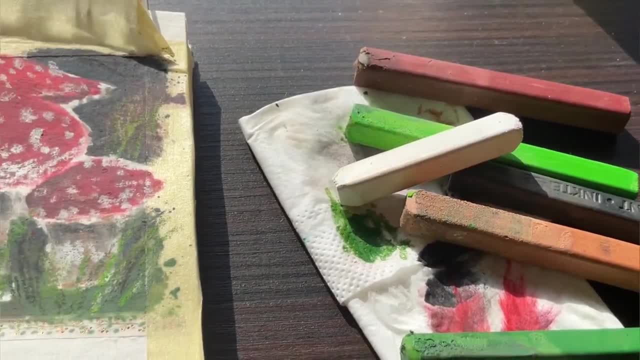 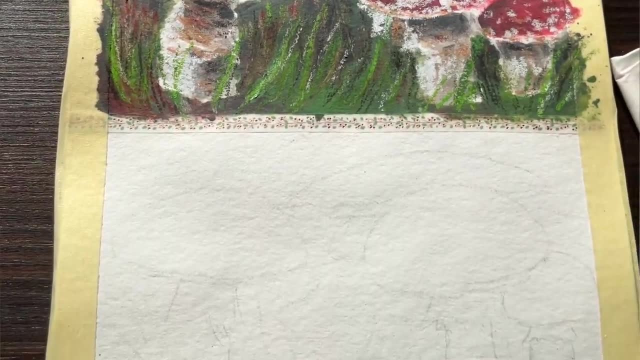 section and I think it's interesting to look at them. but I'm going to leave that to you. I'm not sure if you've noticed, but I'm very proud of my black inktense technology. I have absolutely no problem with it, I'm very proud of it. 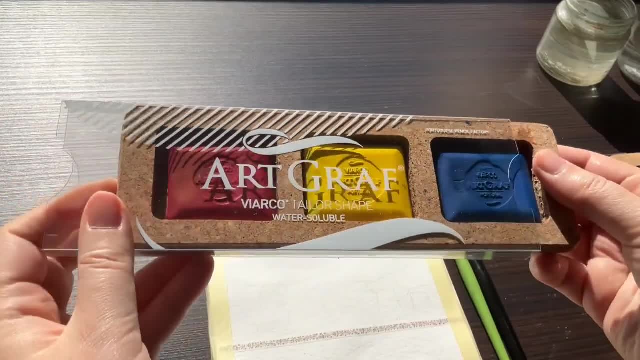 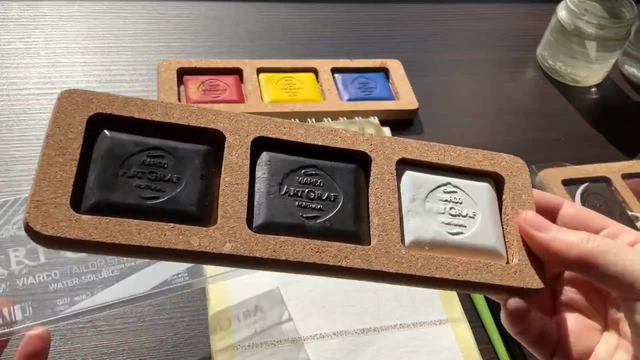 and I want to make the best I can with it. Thank you so much to the second one, which is going to be the artgraph vr code: tailor shapes- painting. i got these tailor shapes about two years ago and boy did i go through a roller coaster with these blocks. 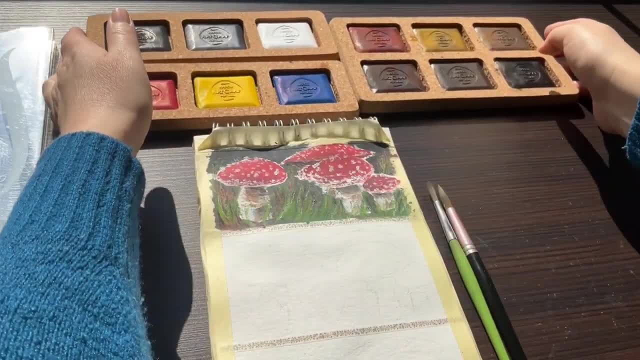 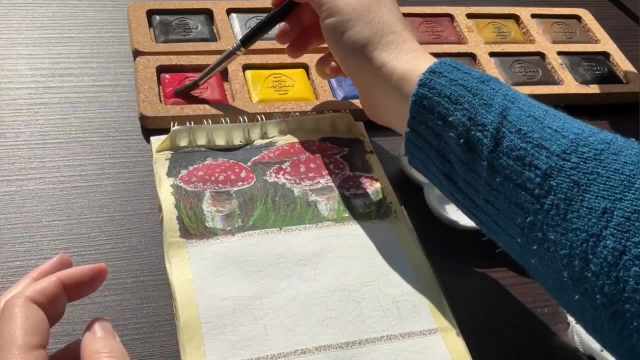 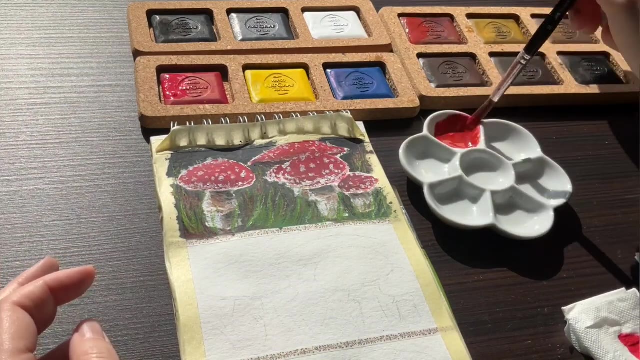 my initial impression in the first couple weeks of using them was love at first sight. then i started to see their shortcomings a bit more and i really ended up disliking them to the point that i completely stopped using them. now i'm in a phase of rediscovering them and loving and appreciating. 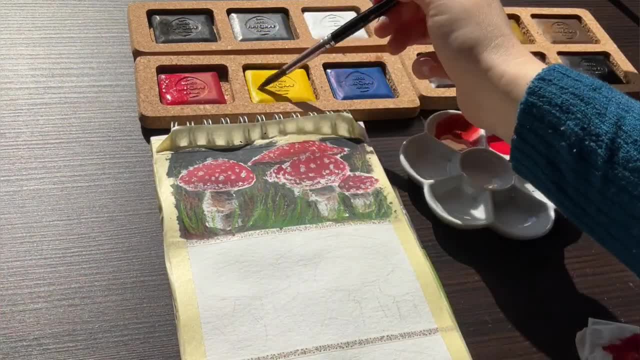 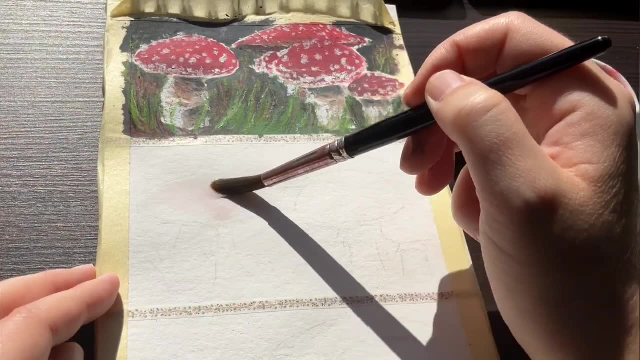 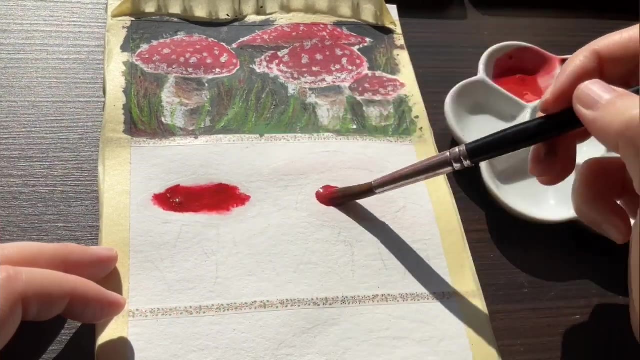 them for what they are. but let's compare them to the inktense blocks first, because i think a lot of people would automatically put them side by side. in my opinion they are quite different from inktense in every way possible. first thing first, if the grainy and streaky ugly face of inktense 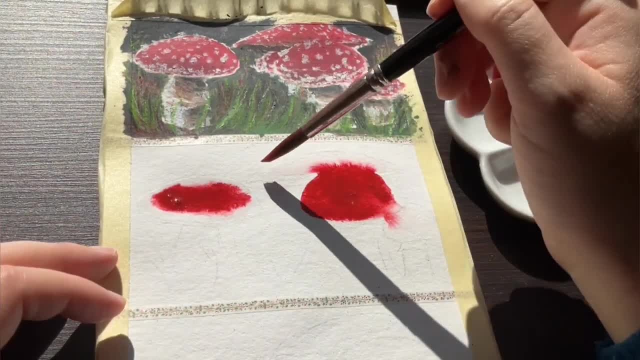 bothers you. you don't have to worry about any of that here. the artgraph blocks are going to be a little bit more difficult for you to get used to, so i'm going to show you a few of them. completely smooth, kind of like gouache. at the same time, they dilute really well. 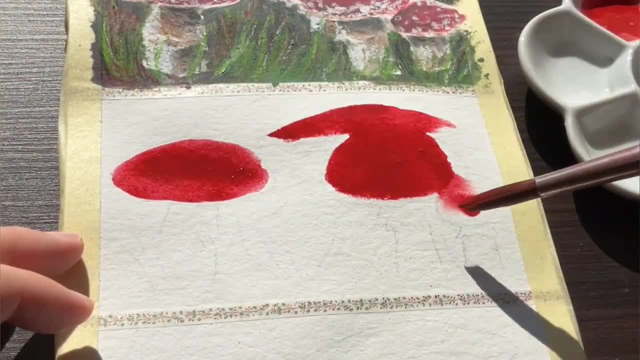 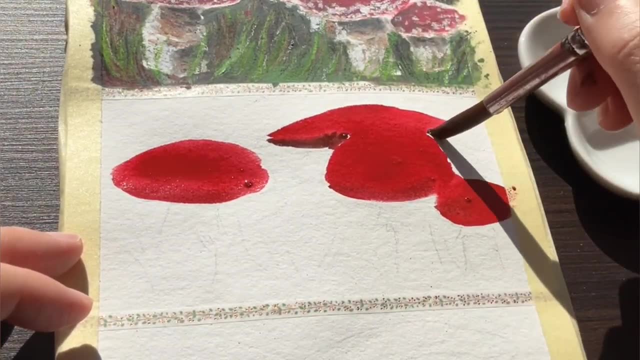 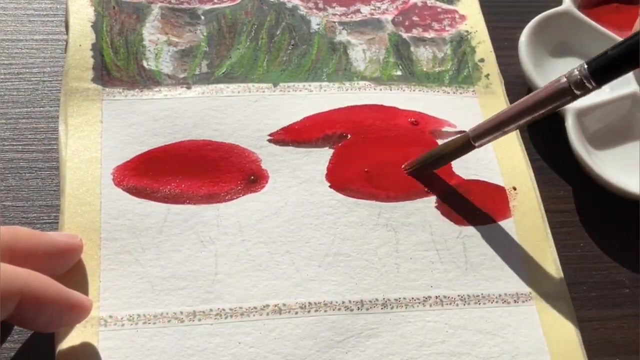 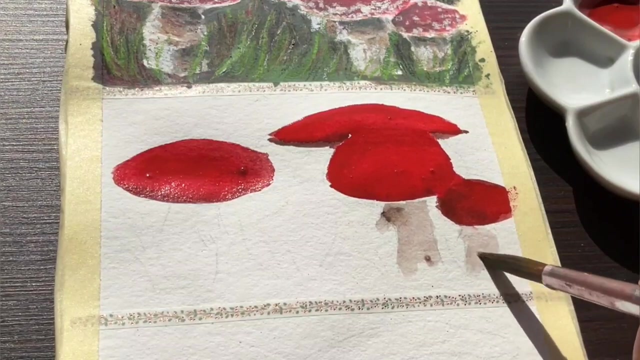 like watercolors and have an incredible flow that is really unexpected from a heavier medium like this one. on the other hand, they have quite a dramatic wet to dry shift that i don't really like and, in my opinion- and this is just my personal opinion- not everyone. 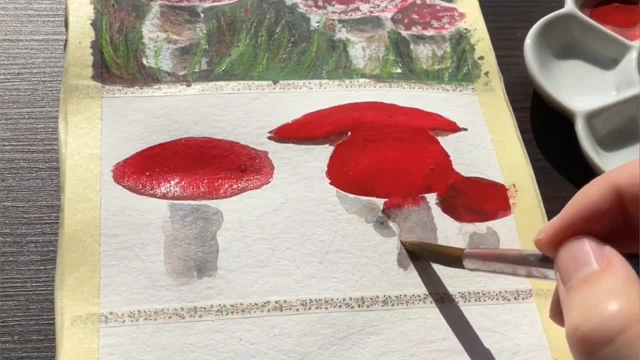 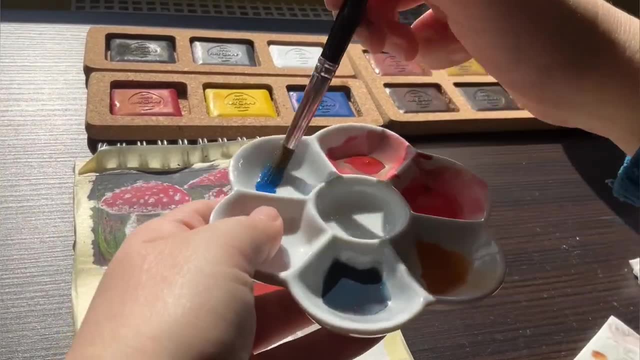 is going to agree. they don't mix as well as inktense and also the selection of colors that they offer in these sets is not very efficient for color mixing in general. for instance, i feel that the 12 count excel intense block set that i used in some of my videos. 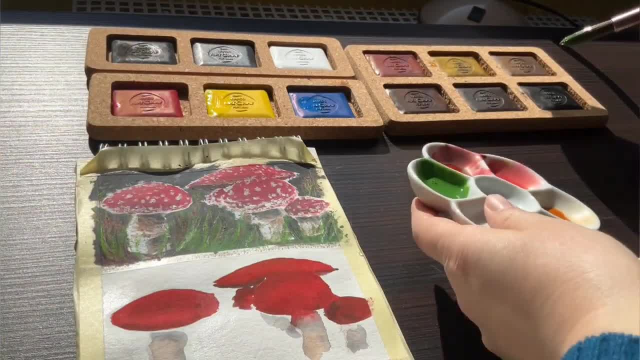 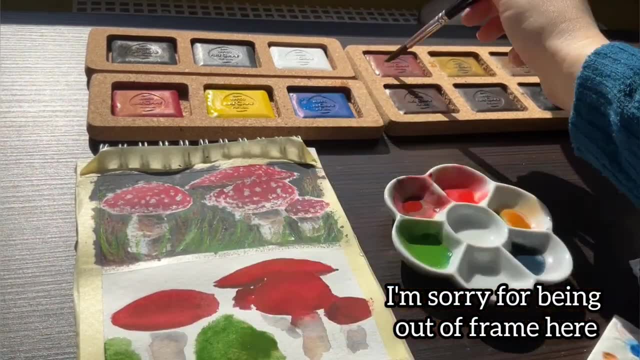 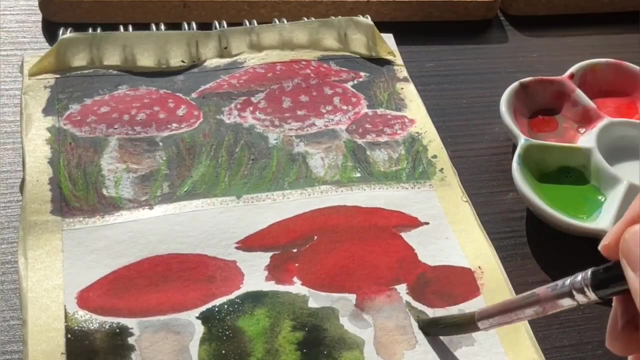 recently, is more versatile when it comes to color mixing and painting with a limited palette. the artgraph blocks have an overall muted feel to them, good for autumn and winter themes, not so much for brighter themes like spring and summer paintings. however, if you enjoy using the derwent, 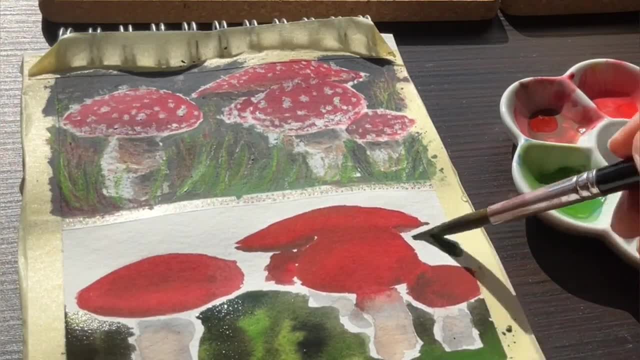 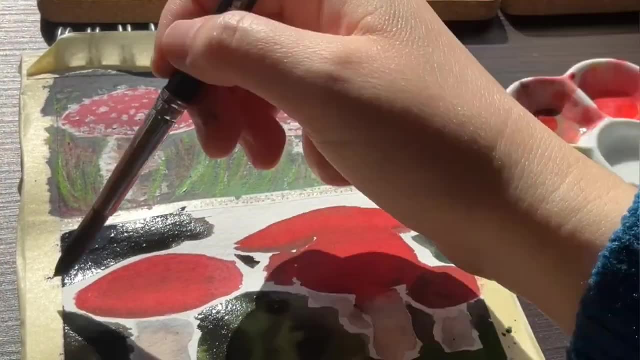 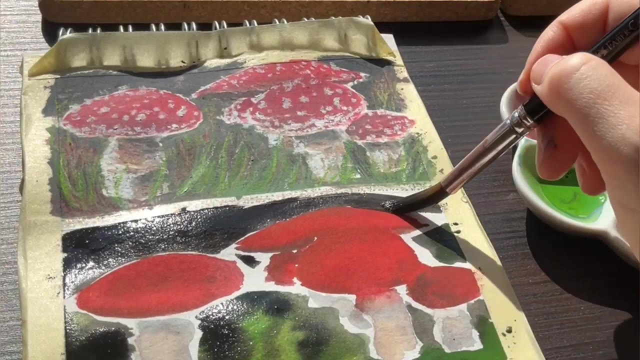 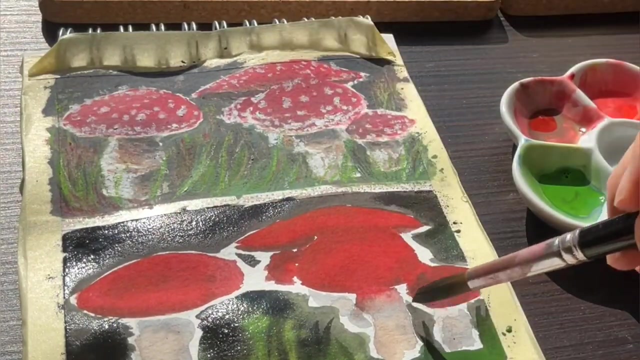 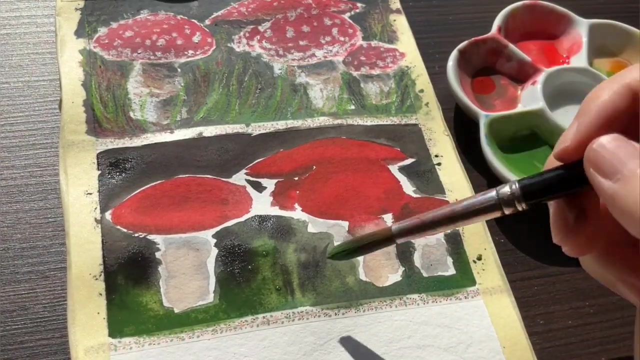 excel graphite and charcoal blocks, which i also do, by the way. this could be an interesting medium to try further your sense of fine flight. much like inktense, the art craft blocks also layer remarkably well and can be built up gradually without any problem. they also don't pull the flower, which is a huge plus in my book. 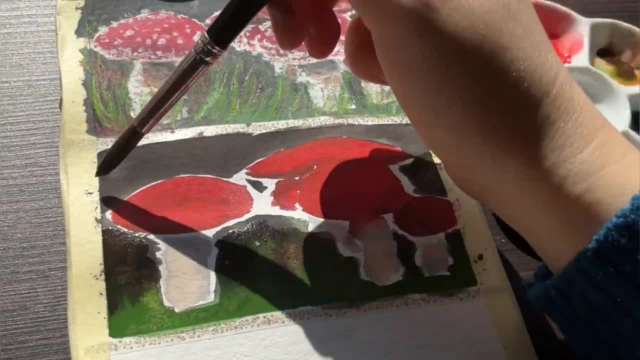 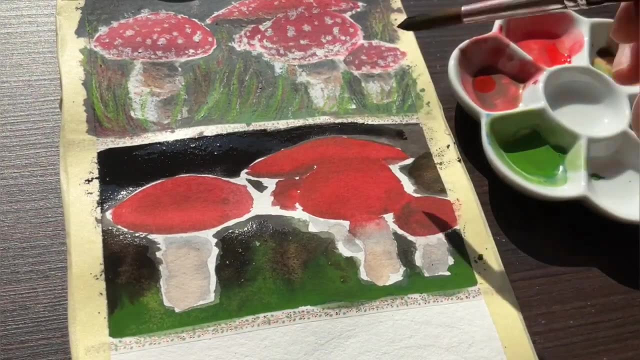 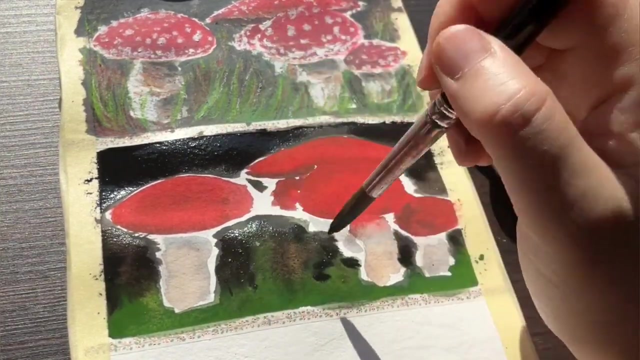 as i tend to use too much water sometimes. in my opinion, it's a very good medium to accompany watercolors. i specifically put together a watercolor palette that I'm planning to use with both the Artgraph blocks as well as the Derwent Graphitint and Charcoal blocks, to kind of bump up the saturation here. 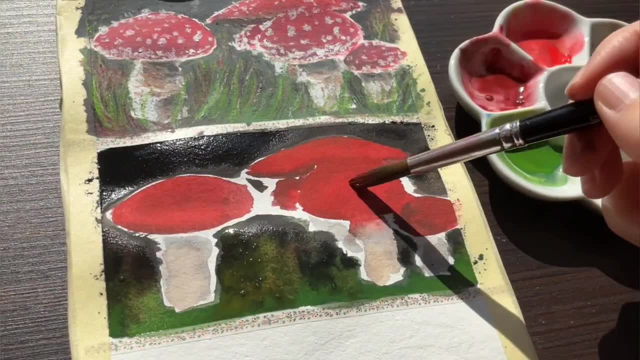 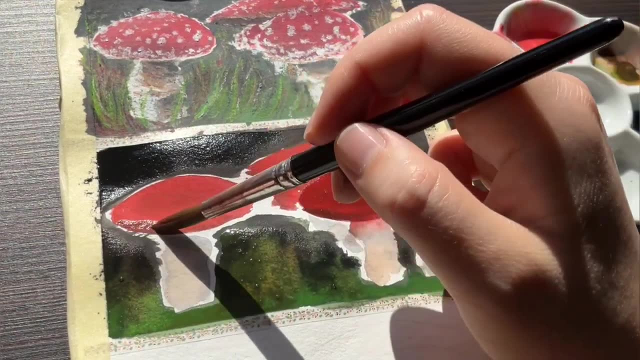 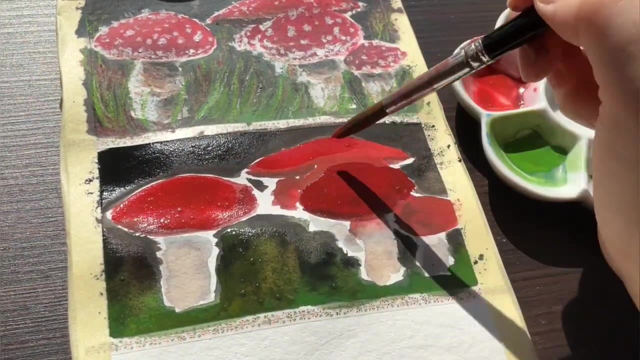 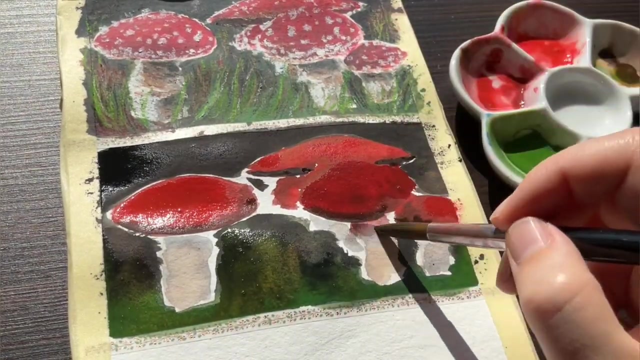 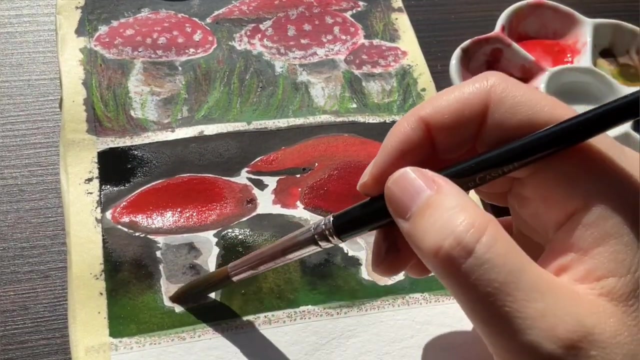 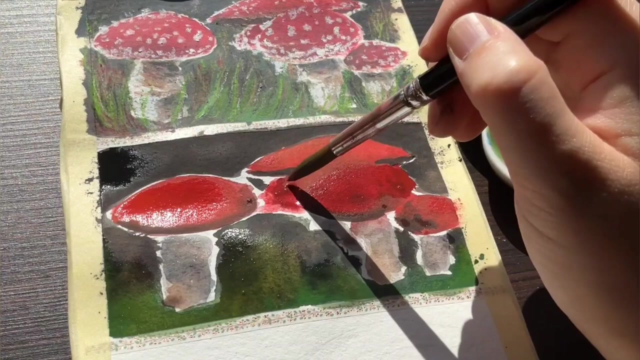 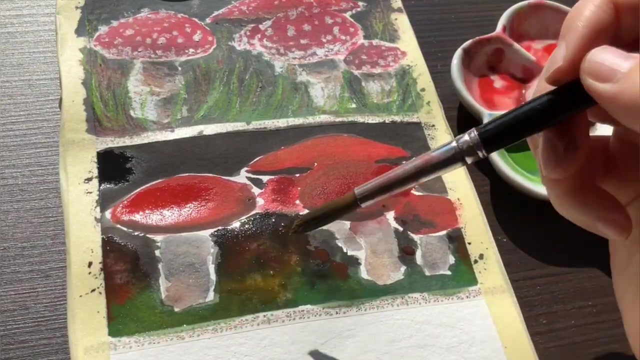 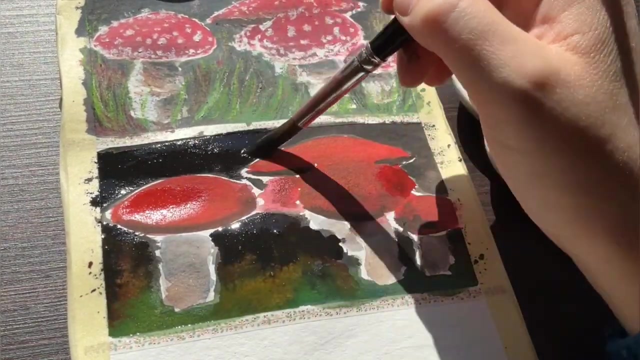 and there I'm planning to feature that in upcoming videos. Another thing that I wanted to mention is that I'm planning to feature that in upcoming videos I'm planning to feature is that these blocks are by far the priciest blocks that I own. You can. 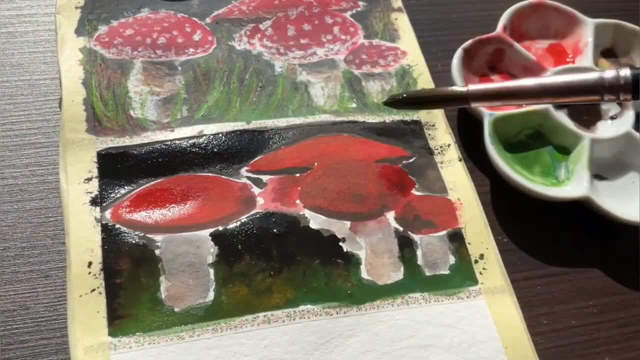 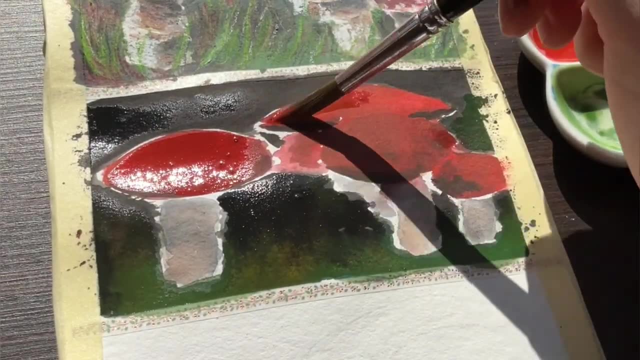 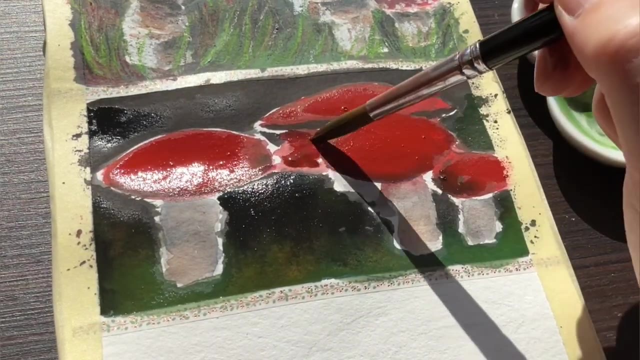 purchase high-end, artist grade watercolors for that money, which could be the reason why I'm a bit more strict with these. I know prices differ in every country and art supplies can become massively expensive due to shipping and import fees only, but these Artgraph blocks are very pricey for me and 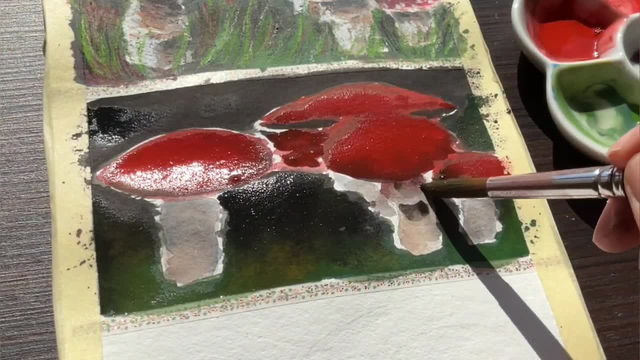 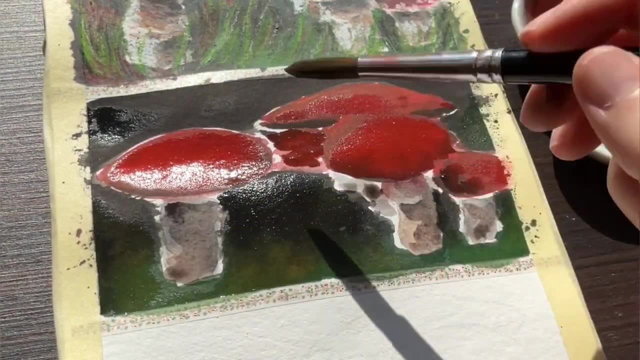 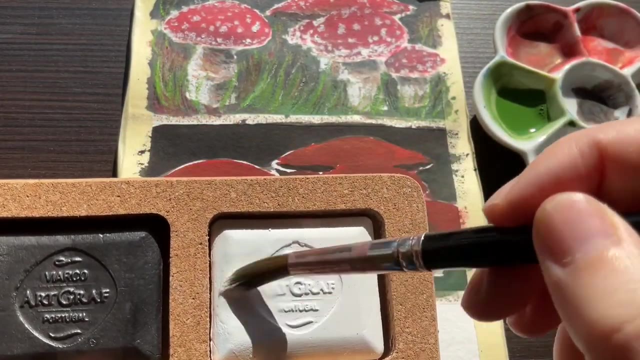 because of the mixed feelings that I have, I'm hesitant to repurchase them in the future, in case I ever run out. But, like I said, I'm currently on a path of rediscovering them and learning to appreciate them. so ask me again a year from now. Maybe they will grow on me and become one of my. 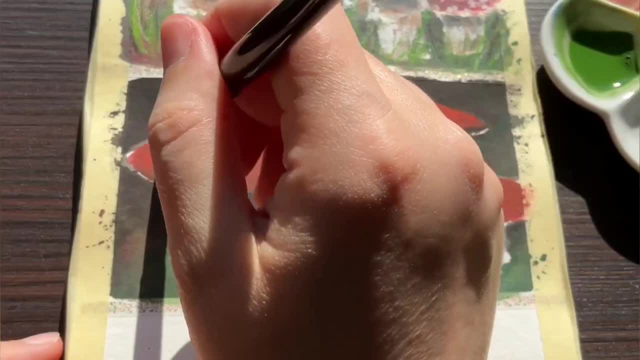 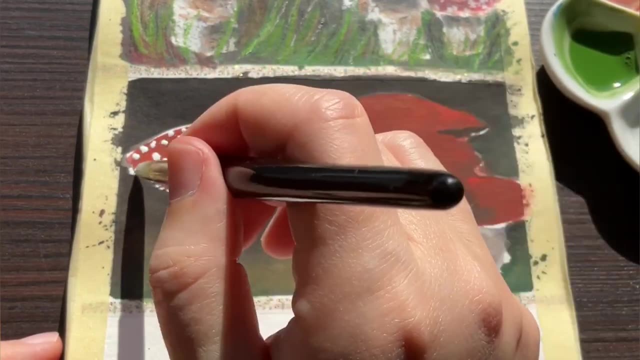 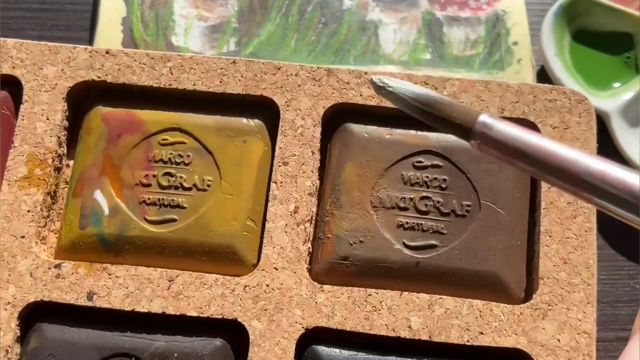 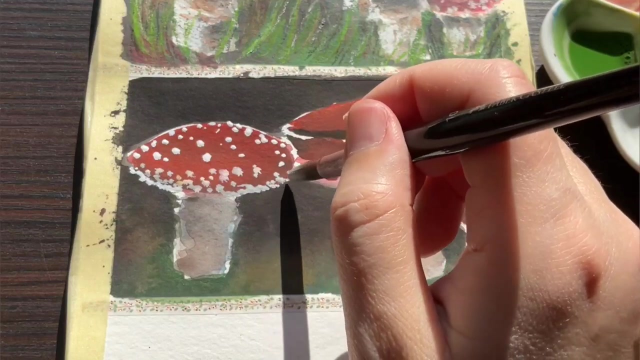 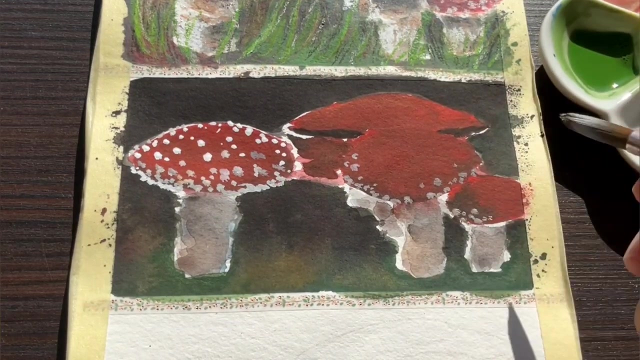 favorite art supplies. who knows If you consider giving them a try. I would say the primary set is a hard skip from me, but the black and white set is insanely beautiful. It's like proper opaque, opaque, white and pitch black, if you like to use that in your art. 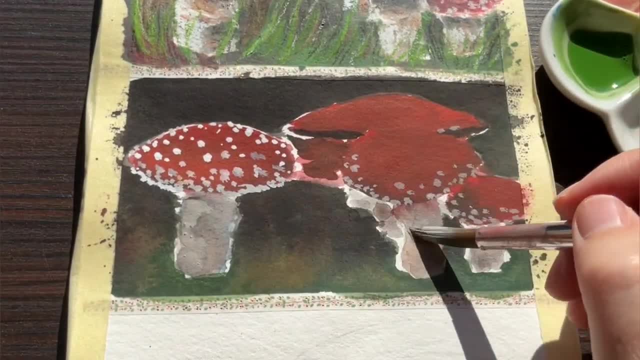 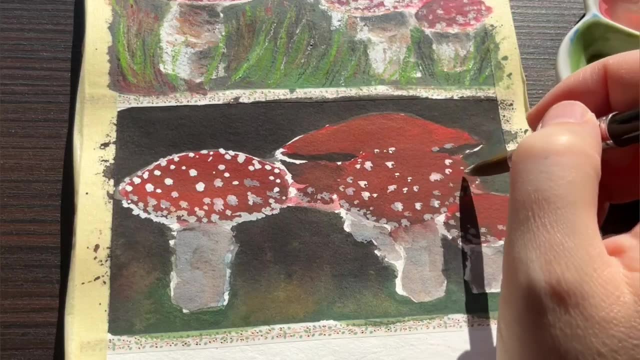 The earth set is interesting. They are a multi-pigment in addition to being a chalk medium, so they don't mix particularly well like watercolors. However, if you want some really punchy, opaque, leaning, really strong earth colors that are often absent in high-end art supplies. 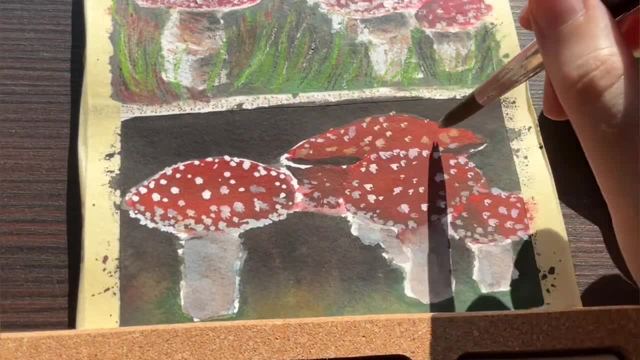 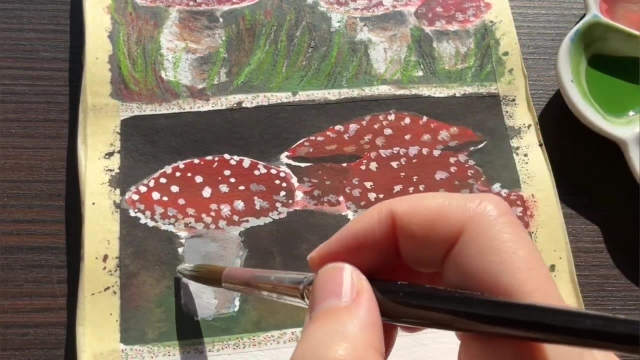 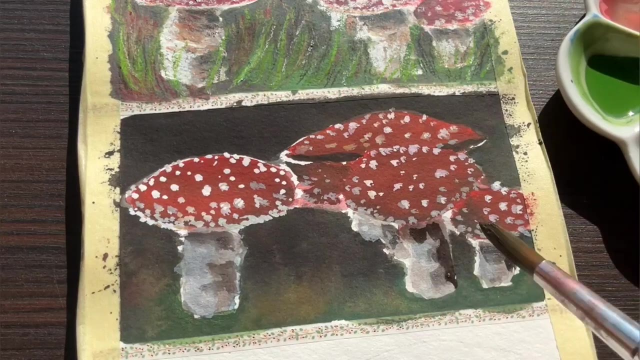 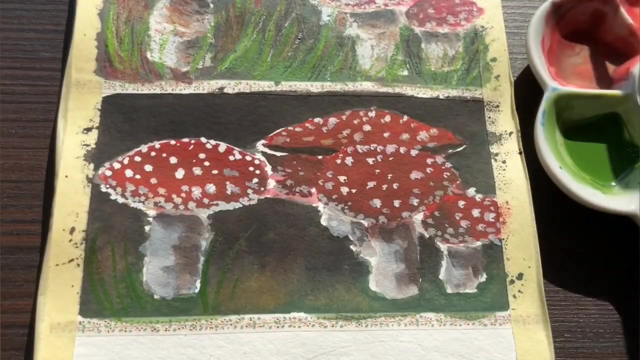 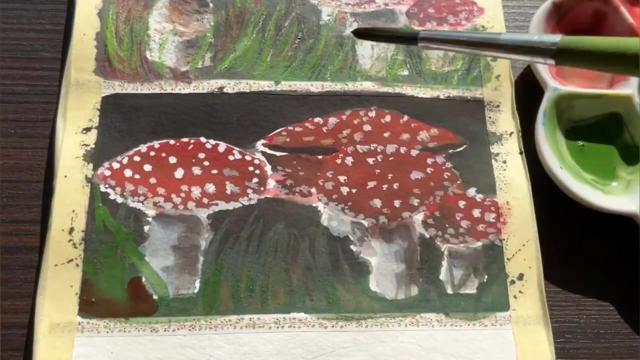 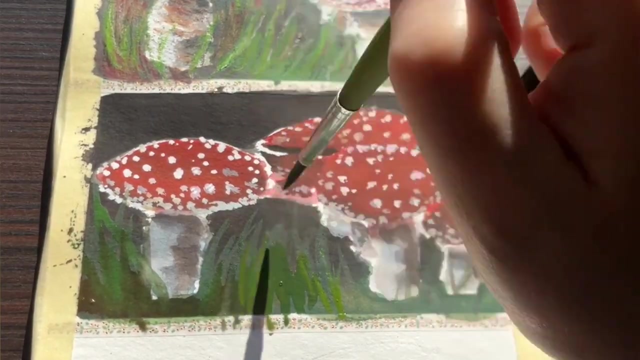 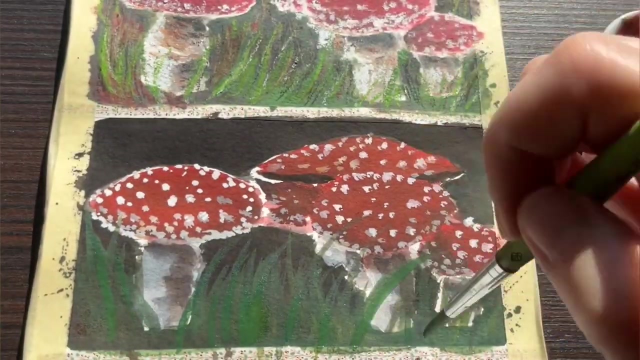 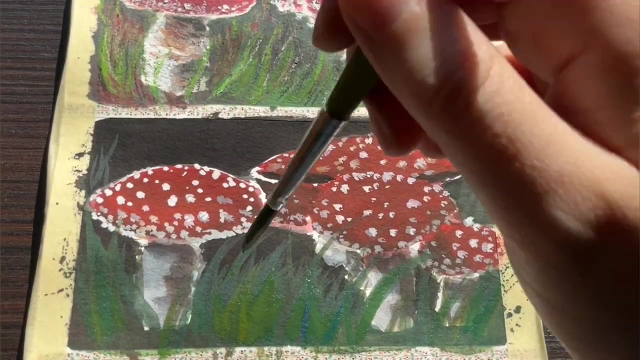 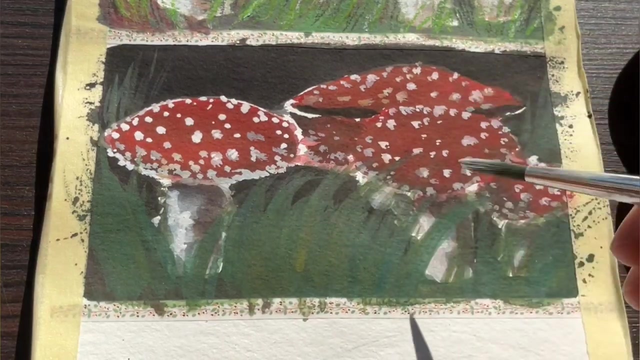 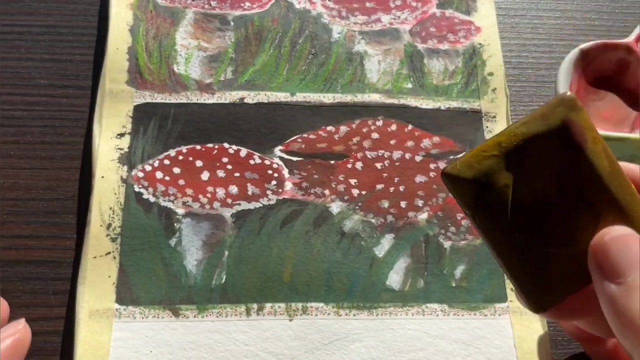 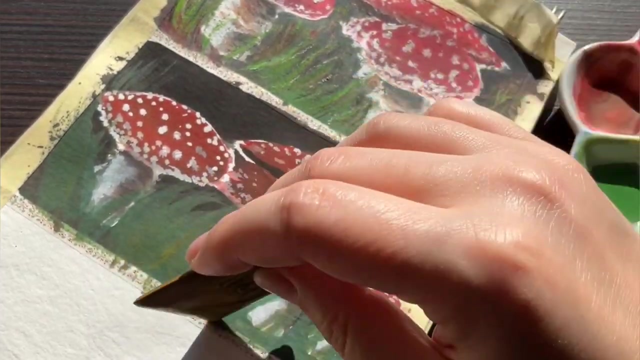 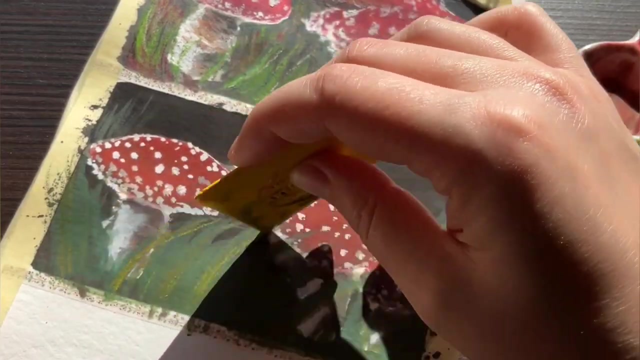 this could be a nice addition. I'm glad that I own the earth set. Thank you. When it comes to drawing with them, they are actually quite hard, not as convenient as the intense blocks, but it is possible to use them that way also. You have to press them down quite. 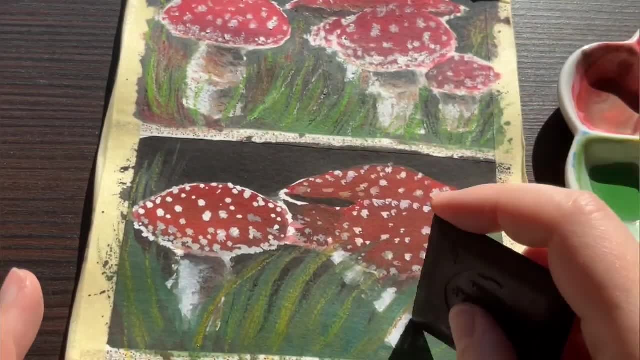 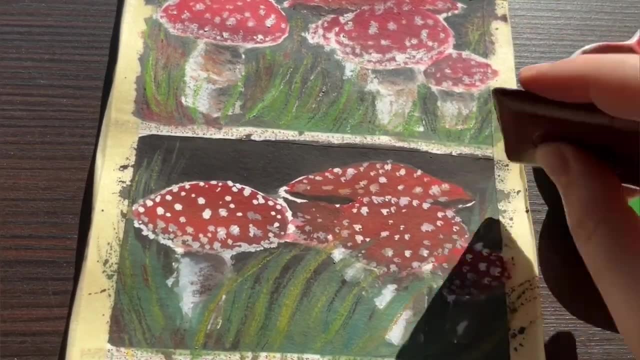 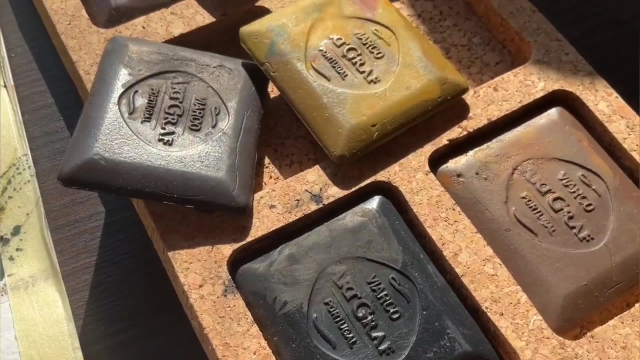 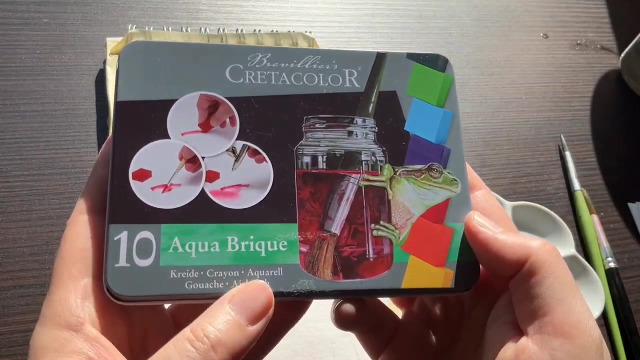 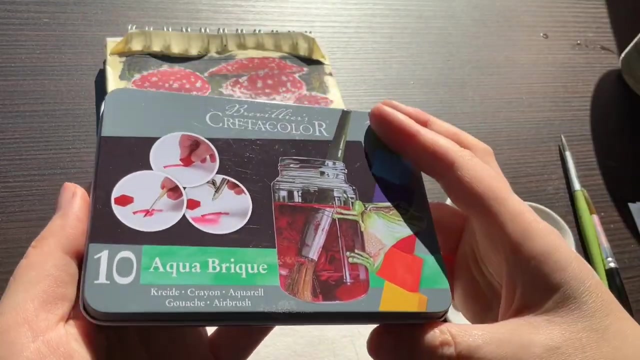 a bit, but they are definitely opaque enough for these kinds of drawings of additional dry pastel effects. I actually really like how this second painting came out. The last product in our comparison video is the Aqua Brick set by Credicolor, an Austrian company that I love for their colored pencils. 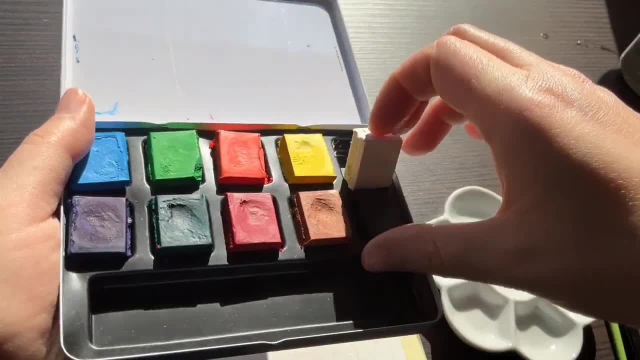 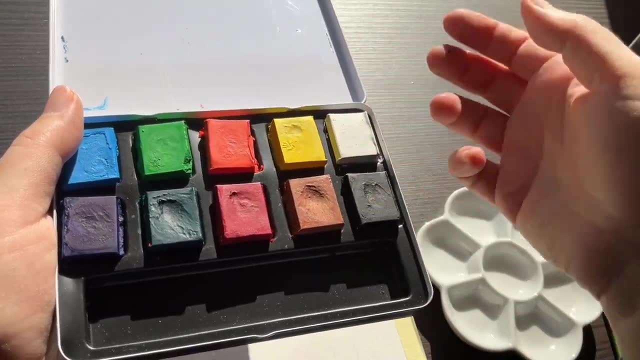 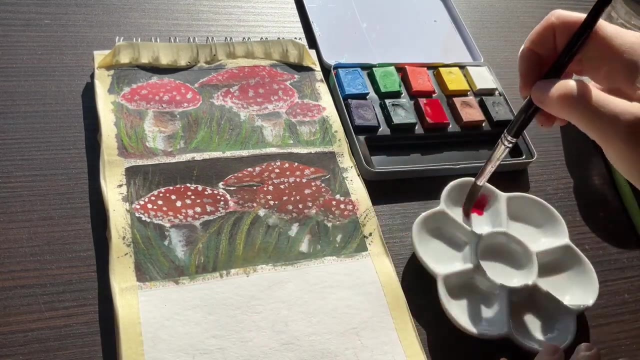 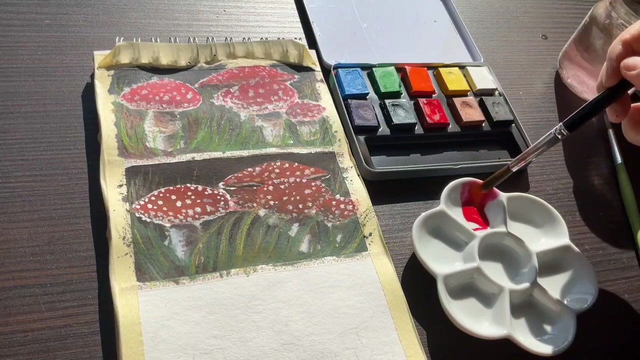 I also have one of their Tinted Charcoal blocks, which is beautiful. I purchased this set last summer purely out of curiosity, because I love Big Man blocks and I wanted to see how this one fares compared to my other ones. It's a very limited palette, probably not ideal for a lot of mixing. 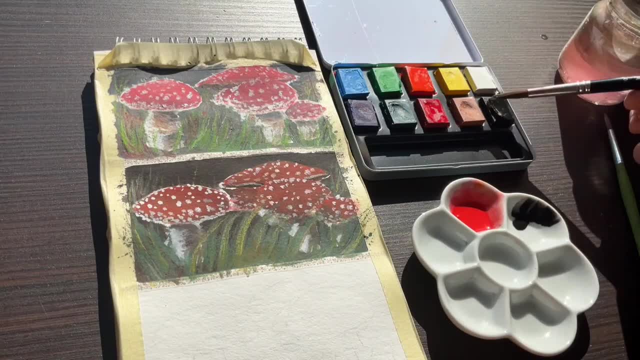 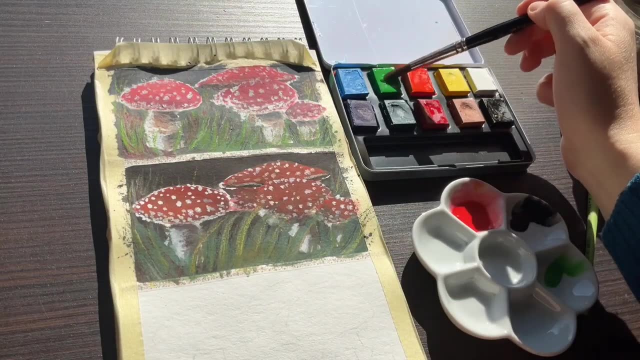 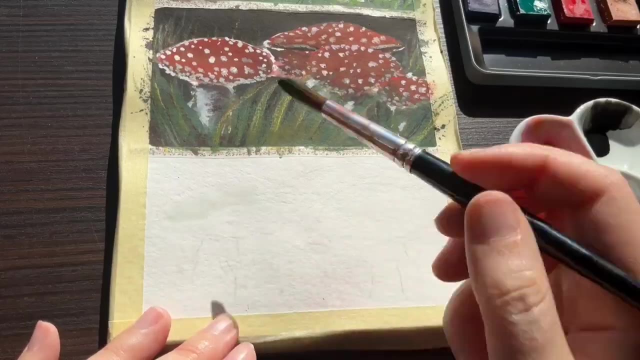 or like realistic paintings. I would say these are some really vibrant, almost ink-like colors that would go really well in an art journal or a mixed media piece that requires a single layer of vibrant underpainting. If I have to describe how they feel when I paint with them, it's basically: 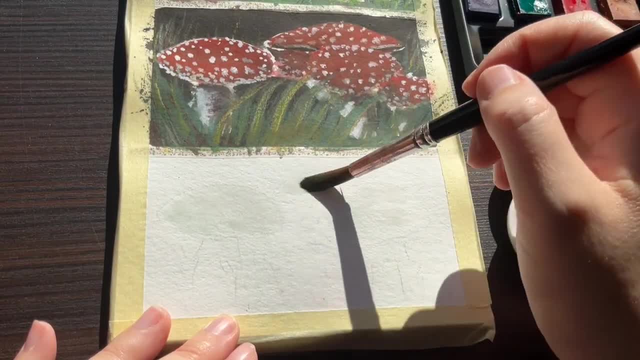 diluted wax crayons like Stabilo Woodies or Neo Colors with like a visible waxiness on the paper. You know that you're painting with crayons. It has its pros and cons, but I don't think it's a good idea to use them as a base. 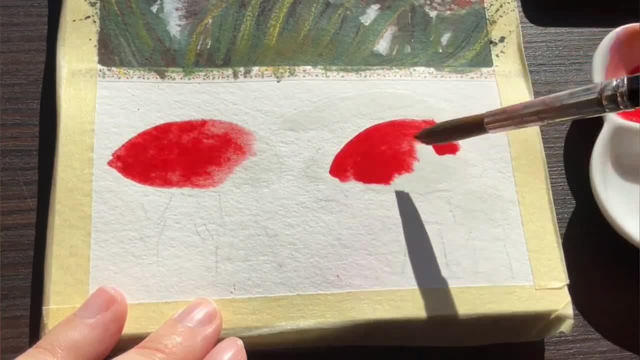 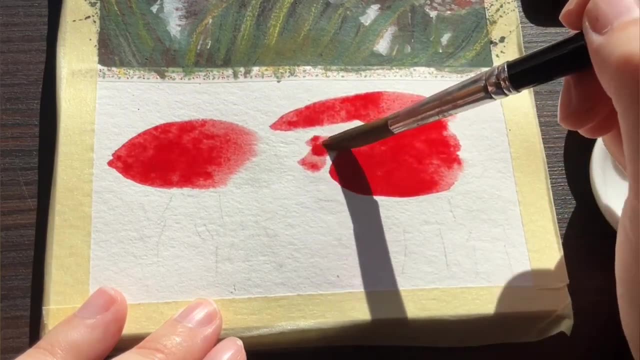 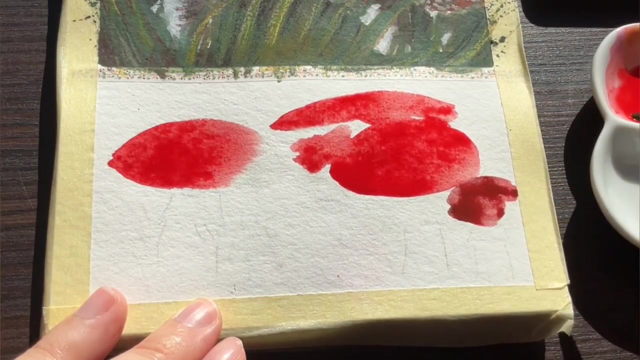 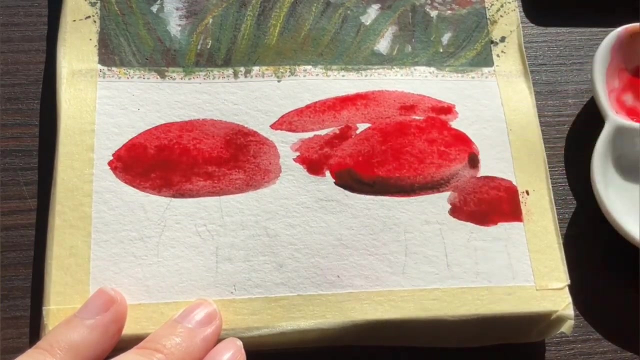 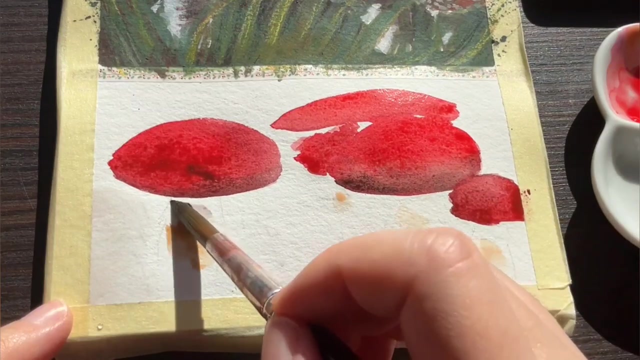 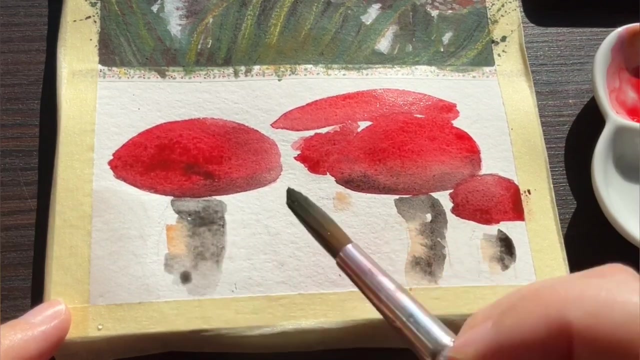 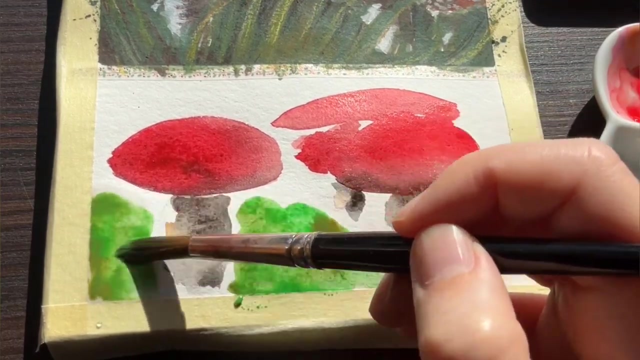 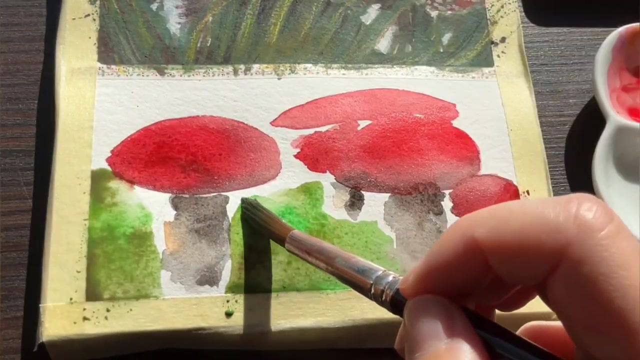 Again, it just depends what you look for in an art supply. Lastly, I'm going to go ahead and call this one Their First Color. You can tell the difference just by looking at it. but I'll say it again, I'm going to go ahead and show you some of my favorite colors. 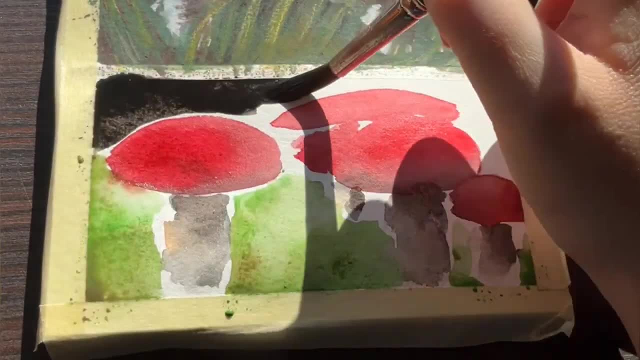 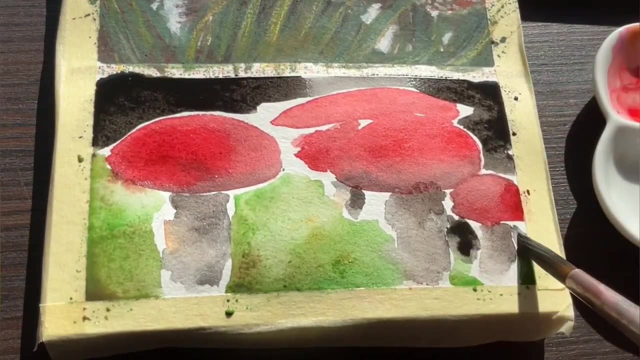 Let me get myself a little cleaner, which I'll do another time. So Carp Acrylic paint. This is a Carp Acrylic paint. I'm going to take a little little bit of paint, Exactly. I have to say, the hues are really, really vibrant and beautiful. 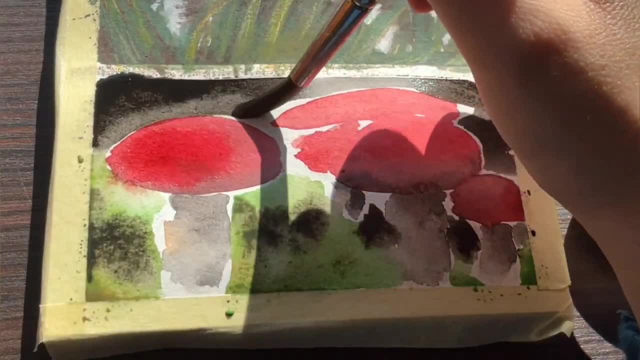 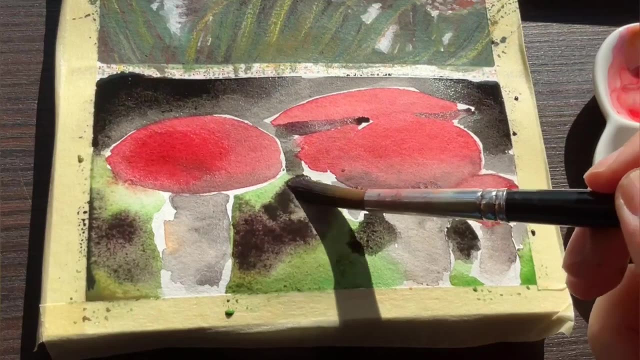 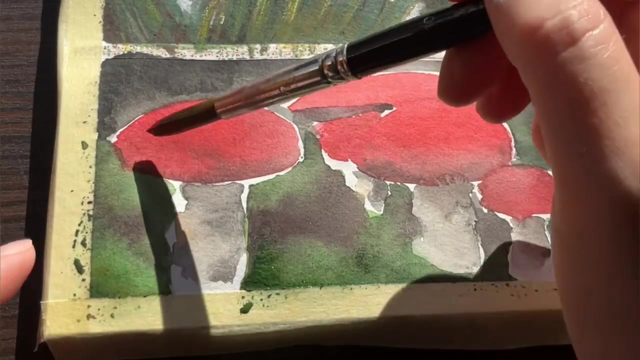 Probably the polar opposite of the artgraph blocks in terms of saturation. These are not realistic looking colors, but maybe that's not what you need in your art. Not everything has to be realistic. I tried to mute them down, though It works to a certain degree and then it just becomes mud, so I tried to not overmix them. 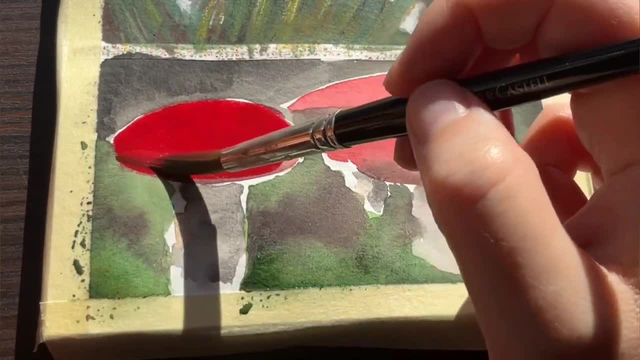 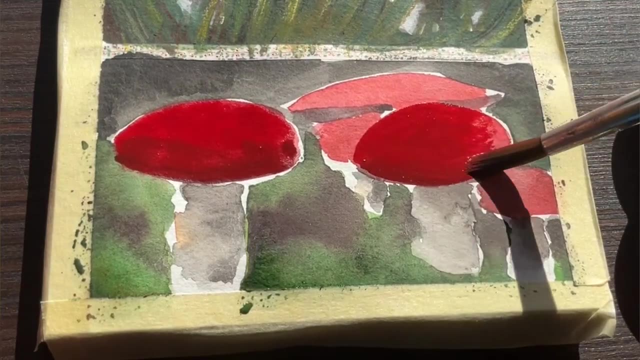 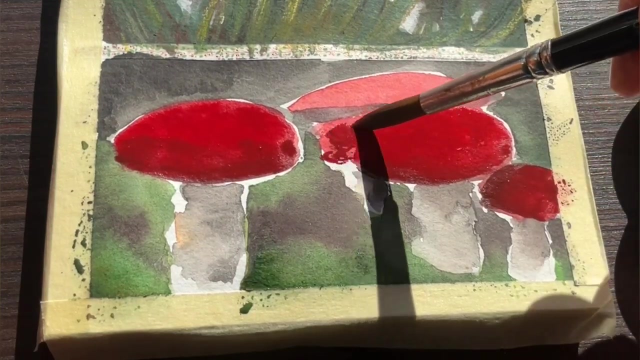 The colors also have a tendency to bloom and to create harsh edges in really wet washes And they do not layer well at all. You have to be extremely careful not to mess up the previous layer. I think I can be honest here and say this art supply is not for me at all. 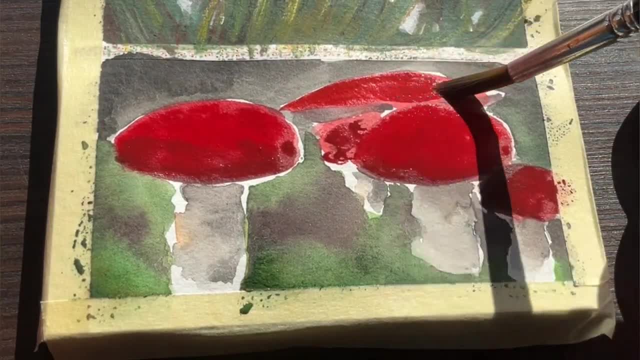 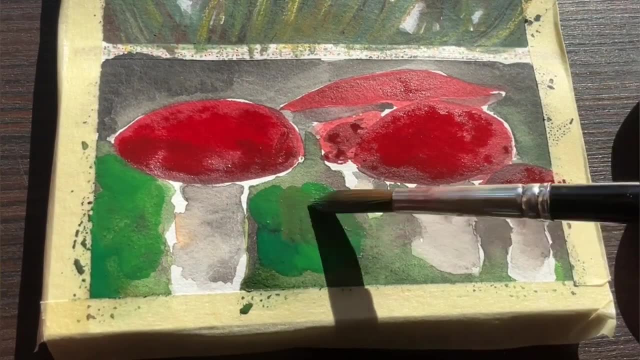 I don't consider this useless, but it simply does not work with my style of painting. I've seen other people use it successfully here on the internet And I saw some very positive reviews on Amazon. so what I'm trying to say is: if you consider, 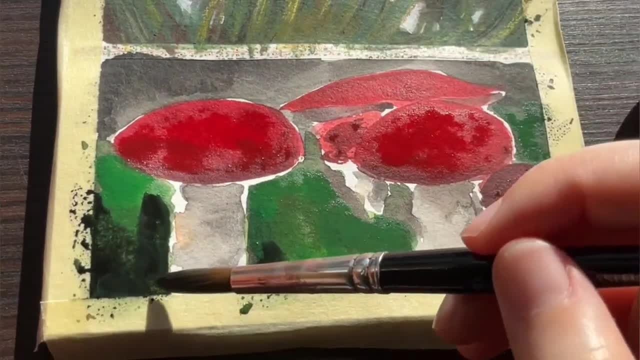 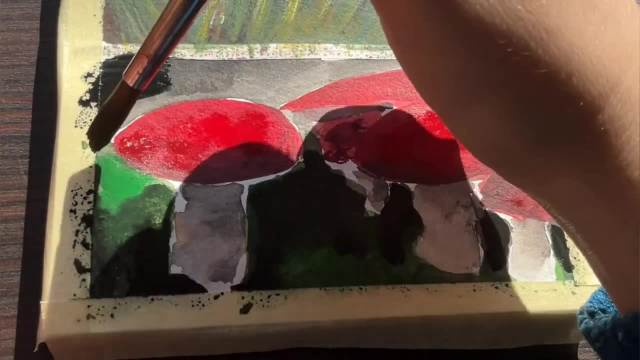 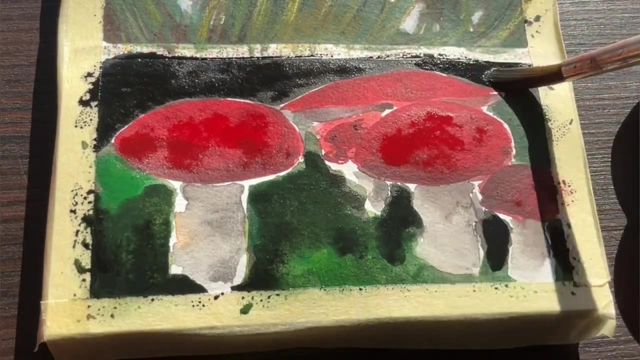 giving this a go. listen to other people as well. As far as this video is concerned, to be completely frank with you, my main goal was to compare the Inktense blocks with the Artgraph VR Co ones, And even though I pointed out a number of differences in many ways- how they behave- 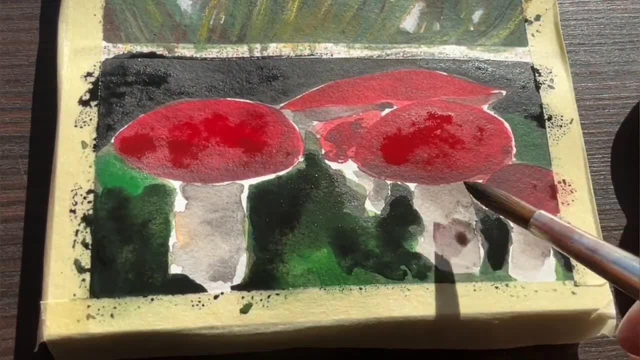 and how they can be utilized. they are quite similar. These credit-color ones are vast. I'm not going to go into too much detail here. I'm just going to show you a few of them. I'm not going to go into too much detail here. 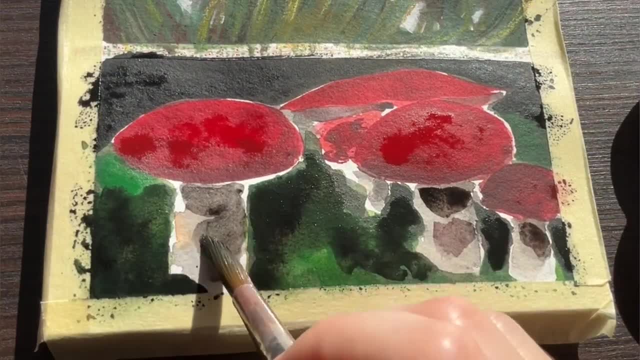 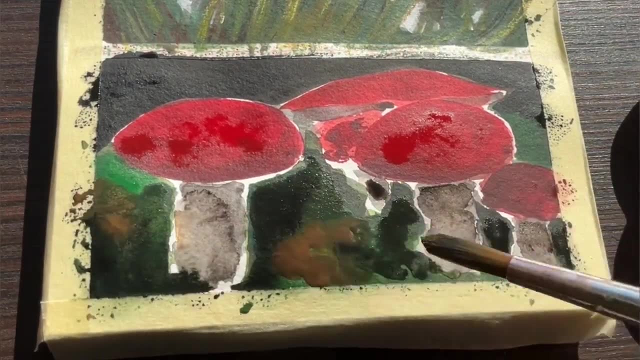 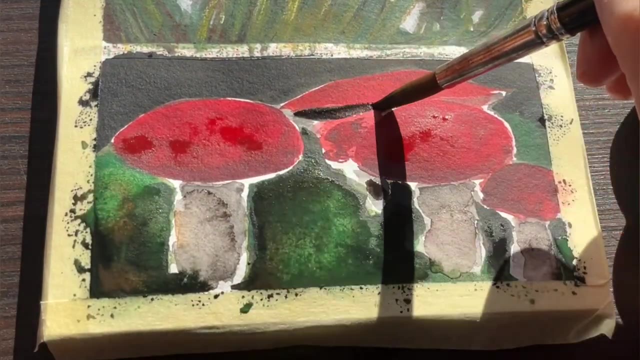 They are technically wax crayons in a block form, so if you enjoy painting with stabilo woodies and neocolors in a diluted form like watercolors, this could be an interesting option. I wanted to include a product that is not along the lines of Inktense, which is my comfort. 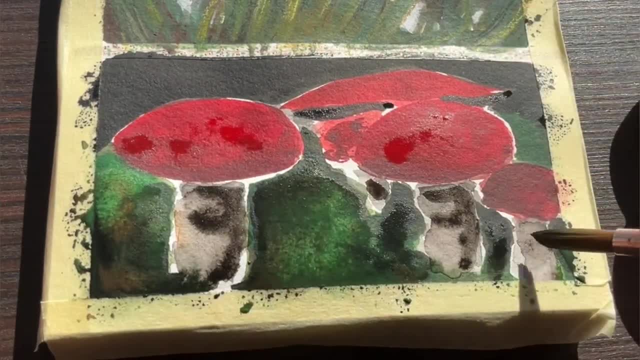 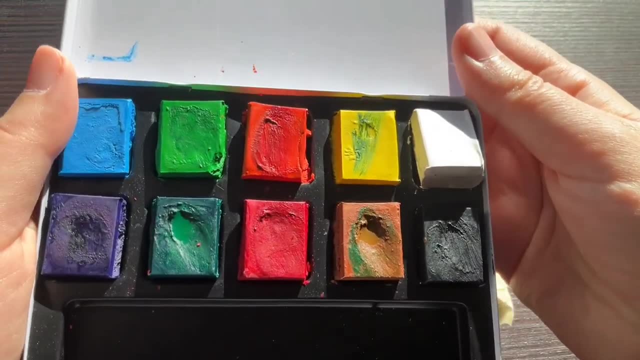 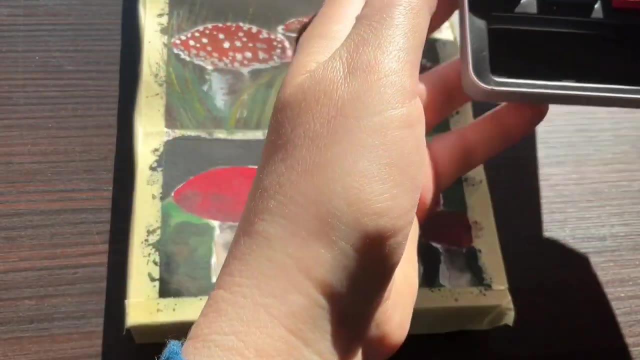 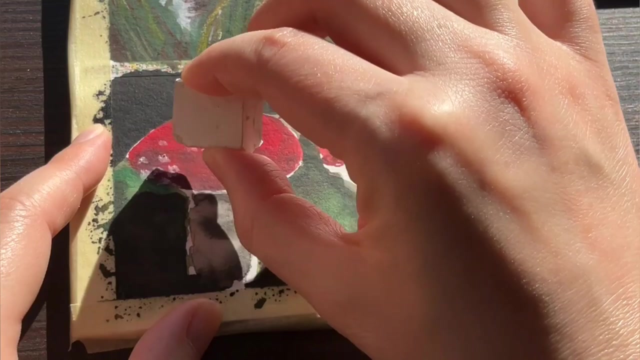 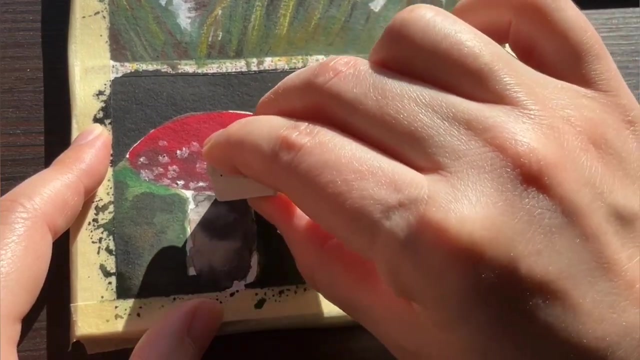 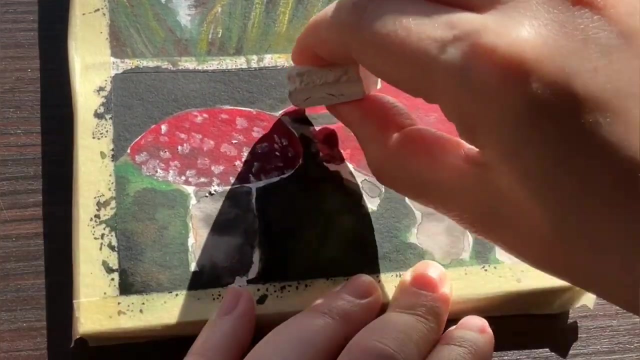 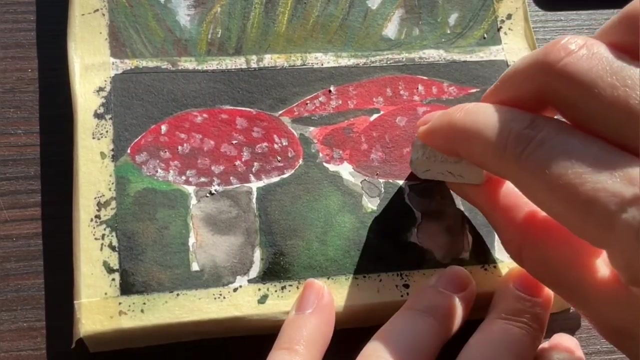 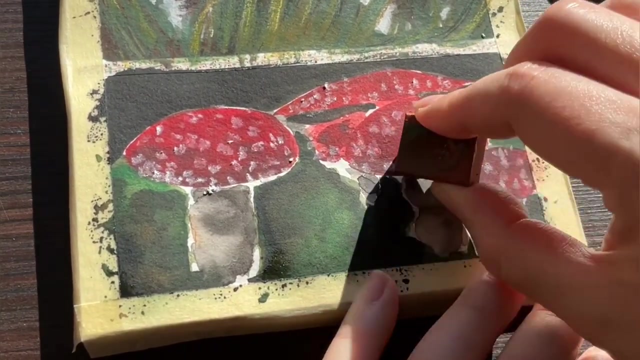 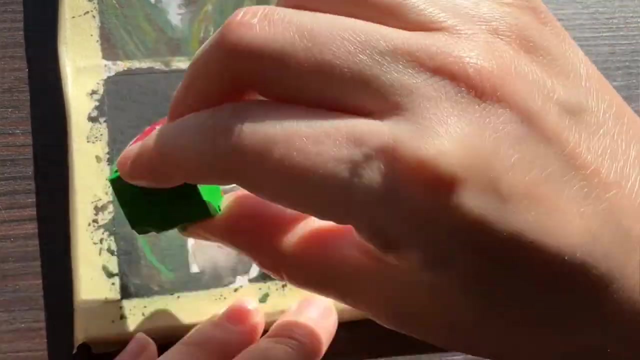 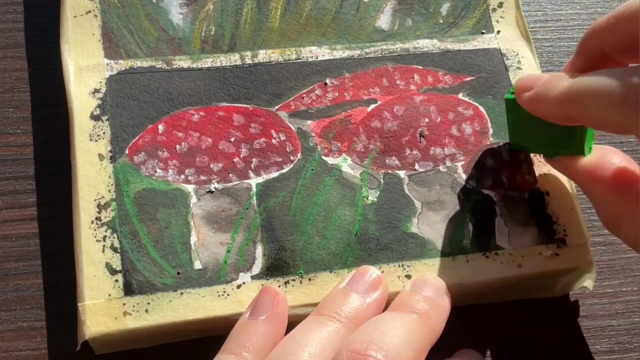 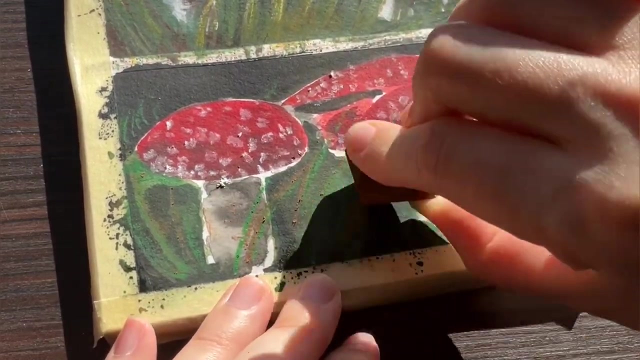 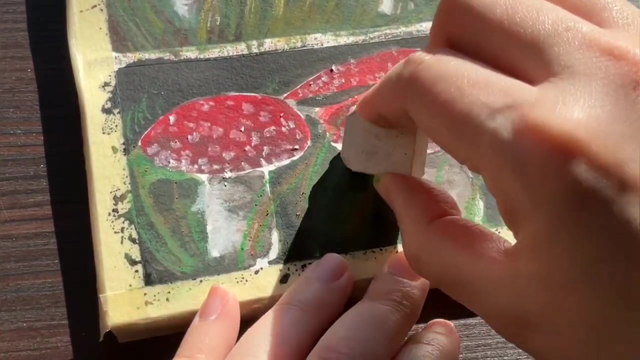 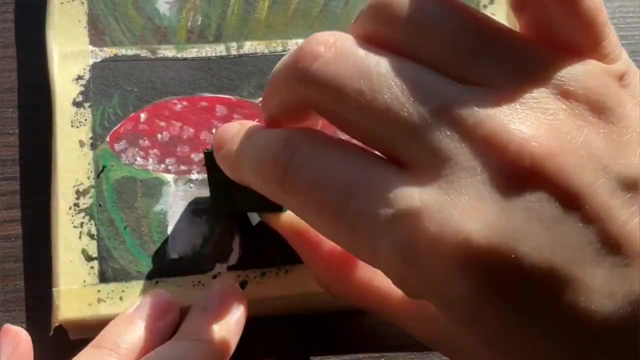 medium in case you really don't like those properties. The credit-color blocks and the Inktense blocks are polar opposites in terms of how they behave, but that's what a comparison should be. Thank you, I really like this painting, up until I started using the box as dry crayons. 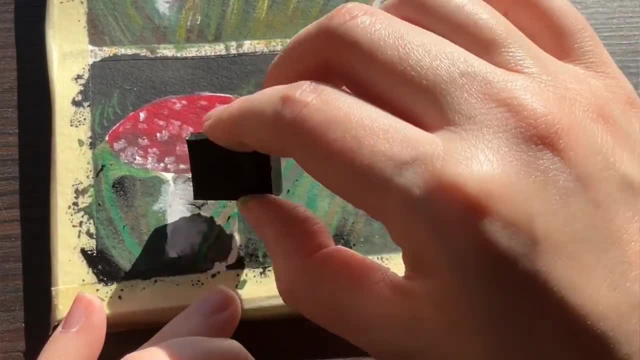 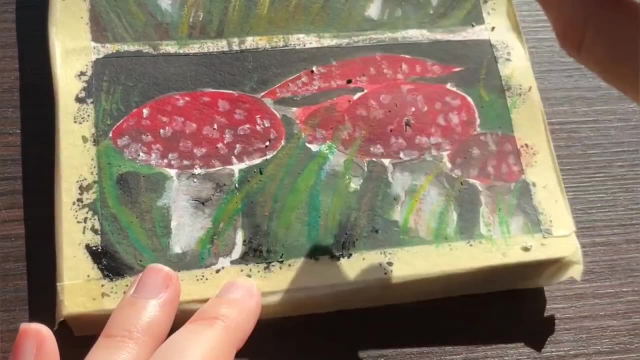 The colors look so vibrant. I loved it, but then it just didn't work. I feel like this third one could have looked a lot better if I had managed to adjust my painting style a bit better to this particular art supply. but it just goes to show it's not for me.